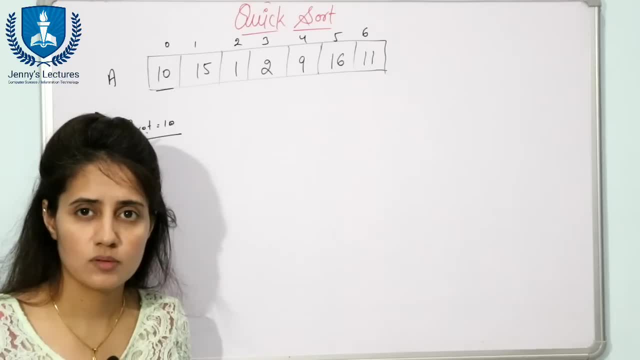 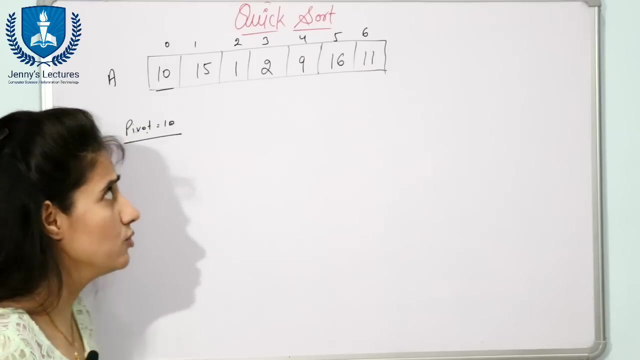 you can say the backbone of this quick sort. okay, that is the main funda, how to partition the array. okay, okay, okay, that is the main funda in quick sort. if you know how to partition this array then you can easily write down the code for this quick sort. okay, now see how to partition this array. now, 10 is pivot. 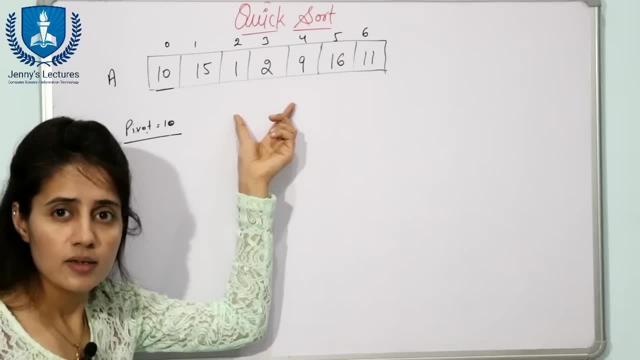 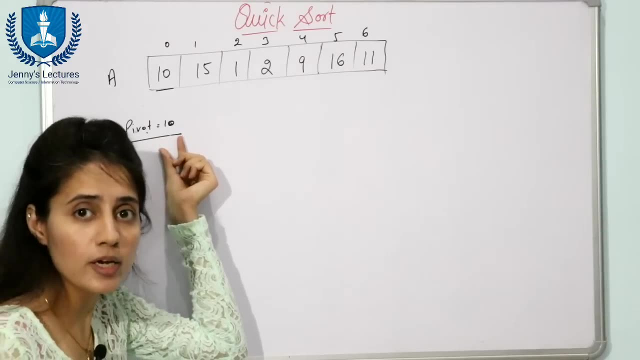 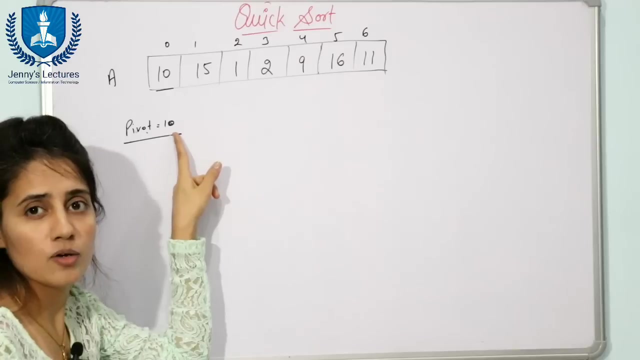 element. now we are going to partition this array in a way such that all the elements less than this pivot element would be to the left side of this pivot element and all the elements greater than this pivot element would be to the right side of this pivot element. okay, and if you know any element, 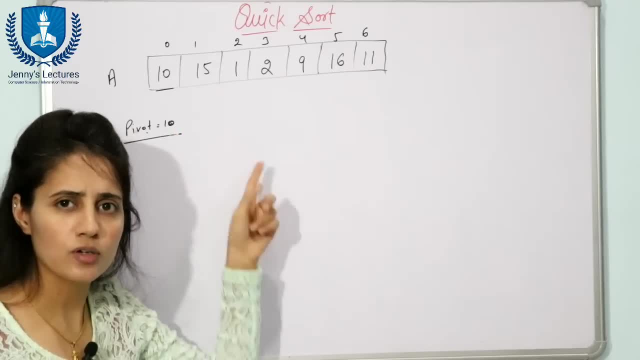 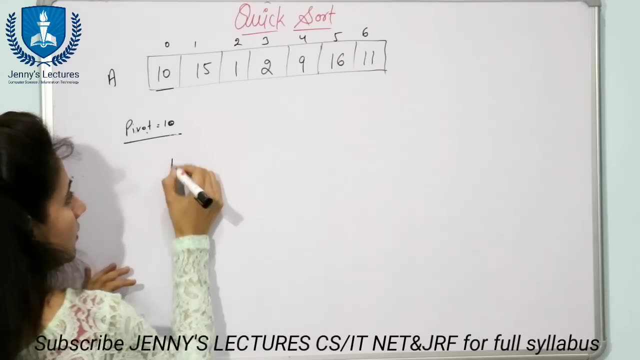 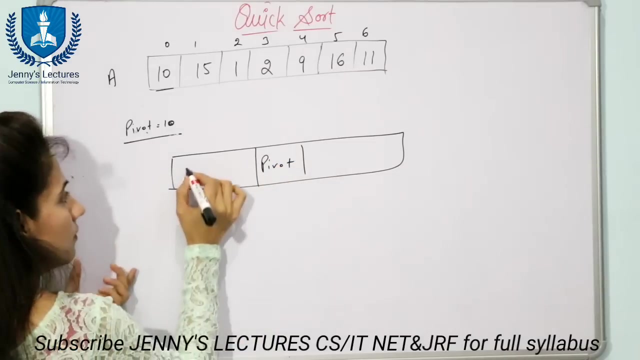 is there which is equal to this pivot element. that element can go either way, to this side or this side, it depends how you are going to implement that logic. okay, now see how to partition this array. after partitioning: see, here we have pivot element, or you can say, key element. this is partition one. 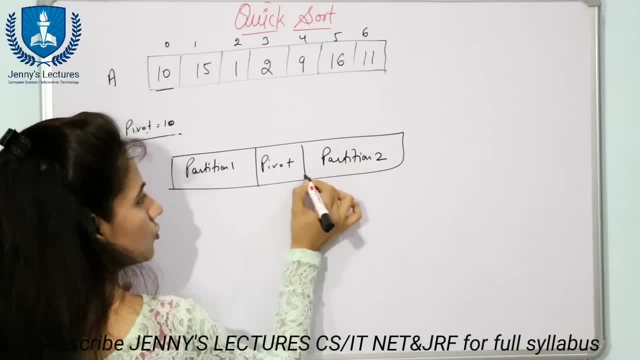 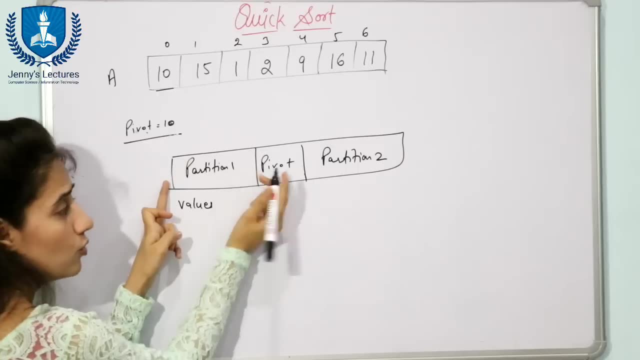 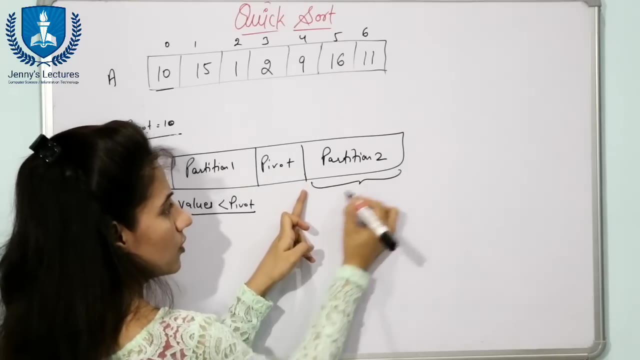 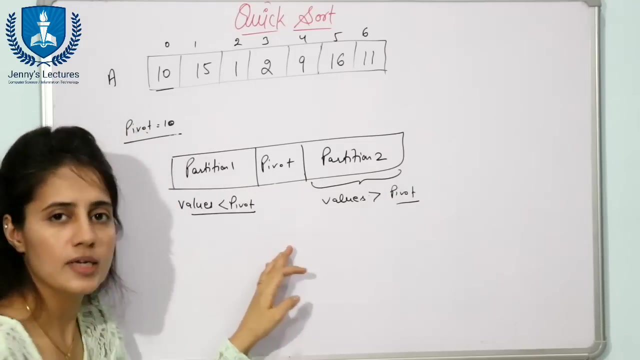 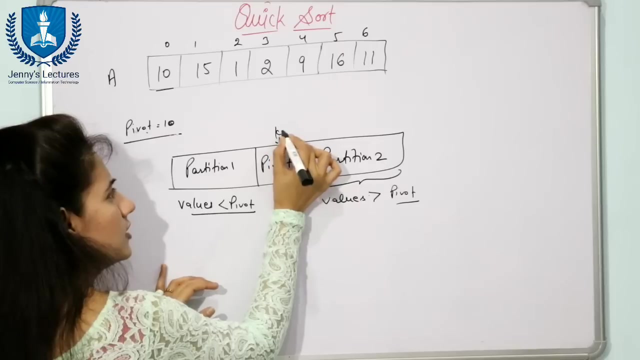 and this is partition two. fine, and all the values, all the values this side would be less than pivot element and these values, all the values to the right side of this element, would be greater than pivot element. equal values can go either way, this way or this way, okay, and this is, or you can say, this is. 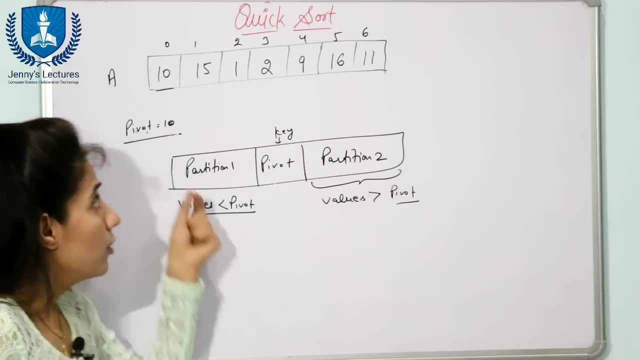 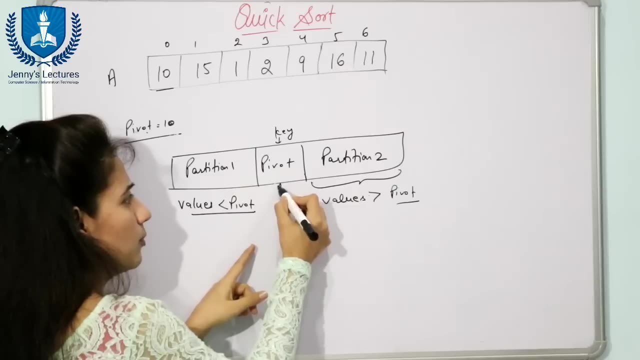 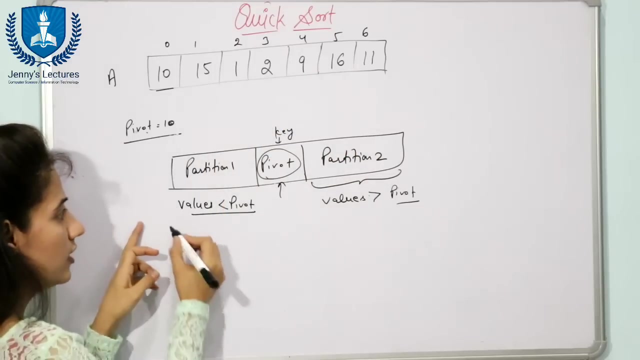 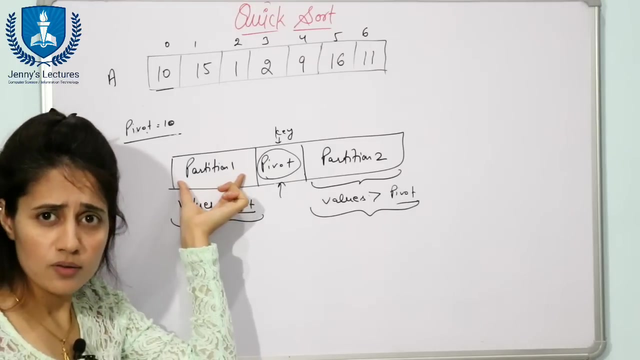 key element. fine, now you have, you have found, you have found out the proper place for one element. right now, this is the proper place for this pivot element. fine, now this. this array has been divided into two arrays: one is this one and one is this one. here the values are i. we cannot say that here. 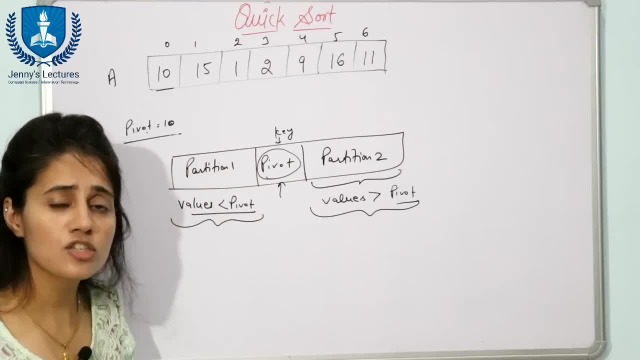 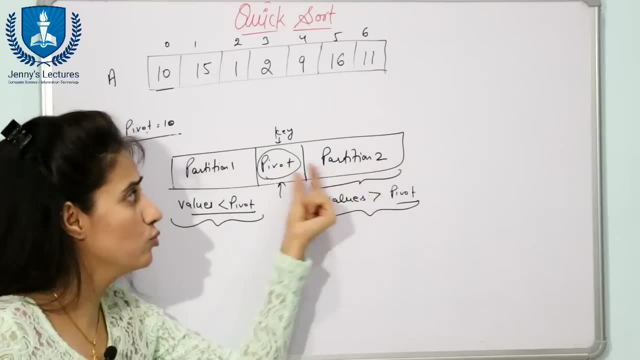 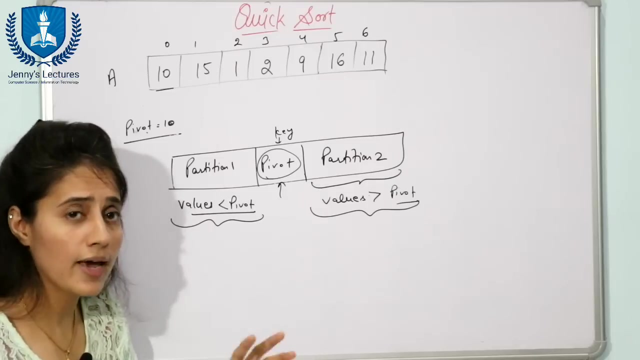 the values are in sorted order. but this is for sure that all the values to this side would be less than pivot element and all the values to this side, to the right of this pivot, would be greater than this pivot element. but we cannot say that, we cannot guarantee that. 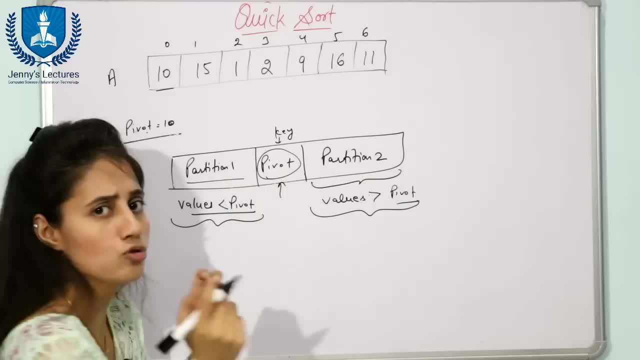 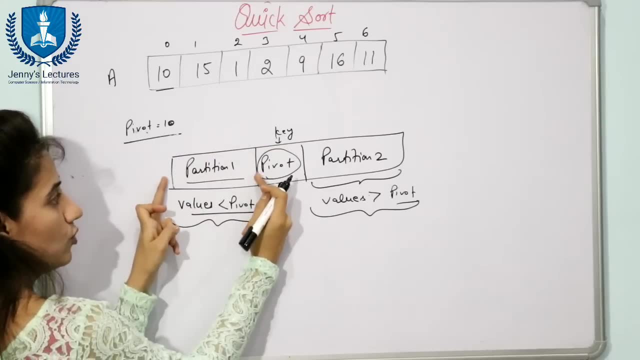 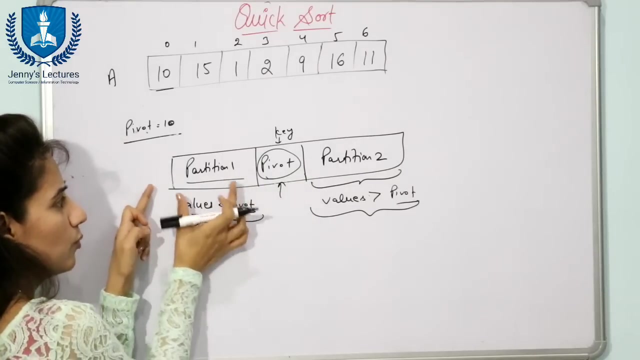 these values are. these values are in sorted order and these values are in sorted order. that is not a case. okay, now, again, again, we will apply. we will apply the same funda to this sub array. fine, and to this sub array. we are going to partition. we are going to choose pivot element. 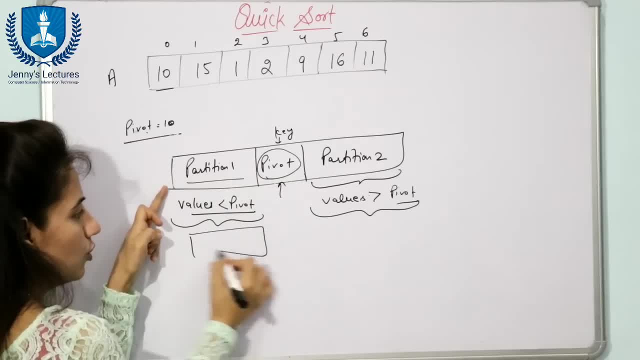 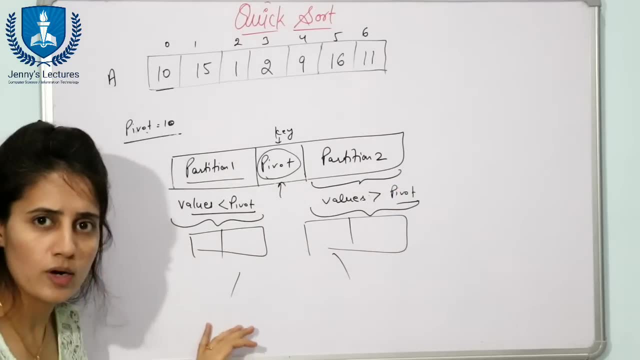 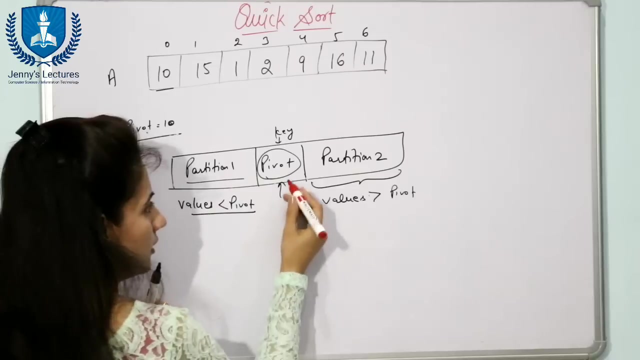 from this sub array. we are going to partition this again into two parts. we are going to partition this again into two parts and we are going to continue this one until we reach, until we have only one element left now. if if you are considering this 10 as pivot element, see this 10 as pivot element. 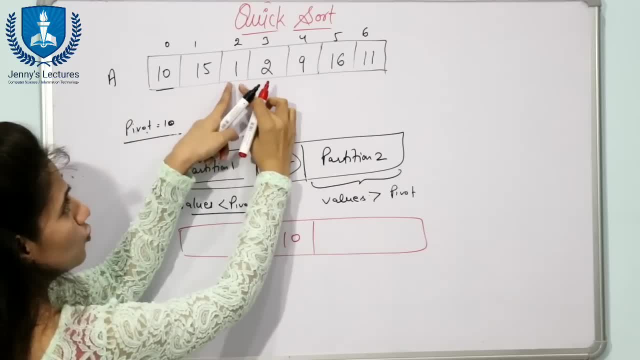 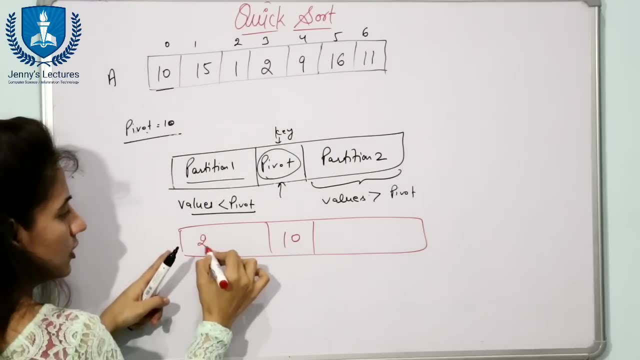 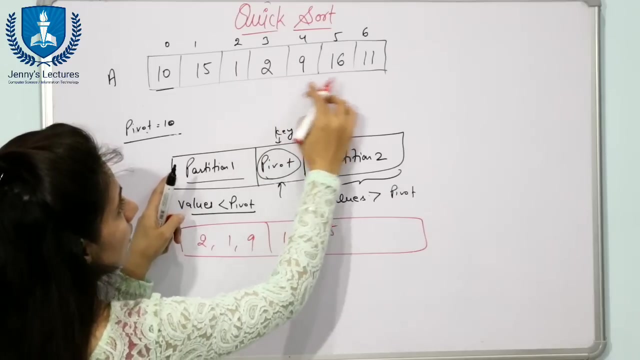 then all the values less than the ten. how many values are there? see, this one is less than this, this two, this nine. so these values would be to the left of this ten. maybe you can say two, one and nine values greater than this ten are, you can say this: fifteen and eleven and sixteen. okay, these values should be to the right of this. 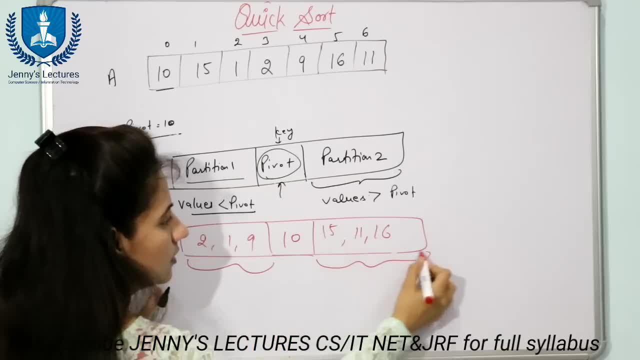 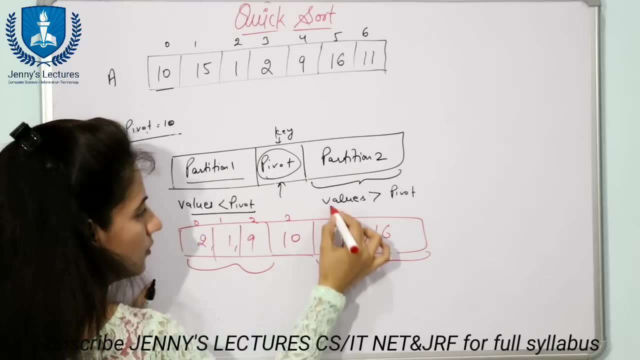 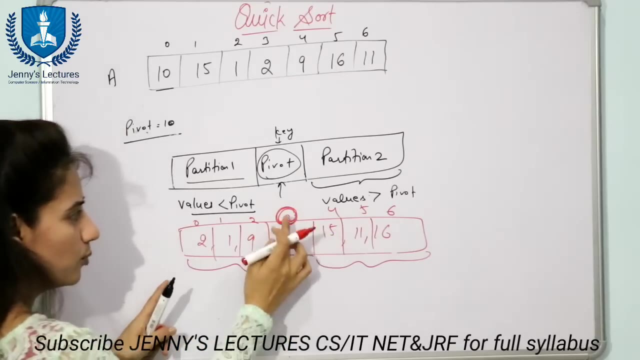 ten. now this is our sub array. this is another sub array. okay, now we have this sub array. okay, so we have five sub arrays. here we have indexes from zero: one, two, three, here we have four, here we have five and here we have six. now see this position, this ten. 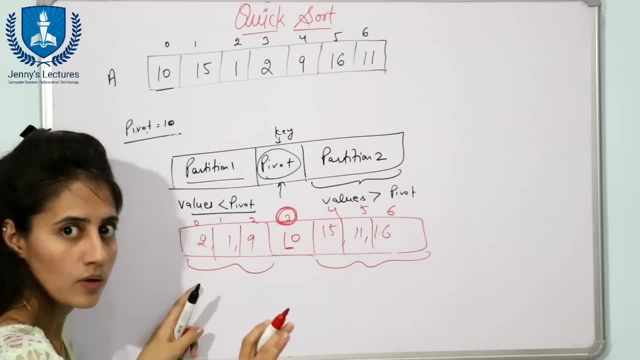 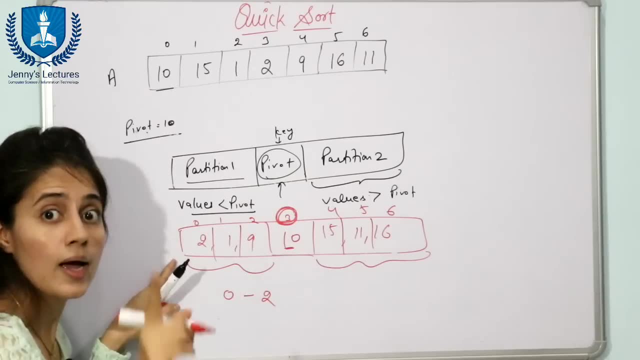 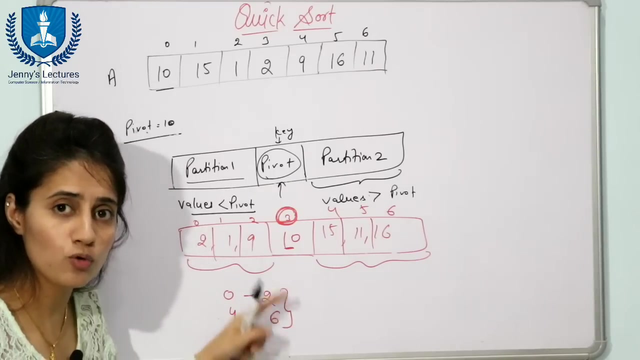 is at position three, so this is at its appropriate place. no need to sort this ten now. now we are going to apply the same processor from And from 4 to 6.. Okay, Regressively, we are going to apply this thing from 0 to 2 now and then 4 to 6 now. 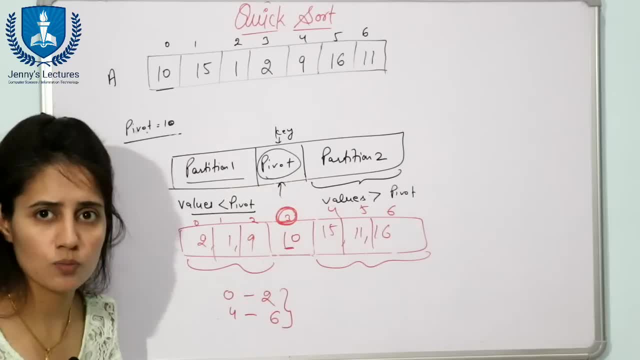 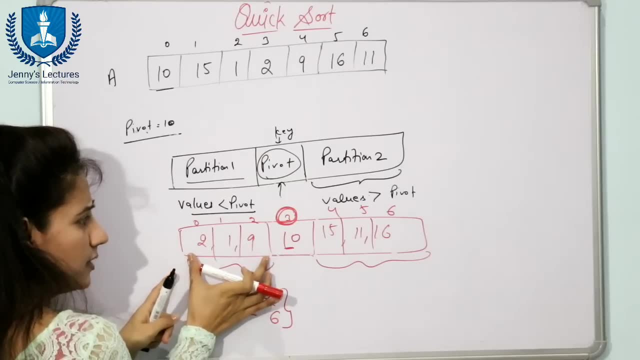 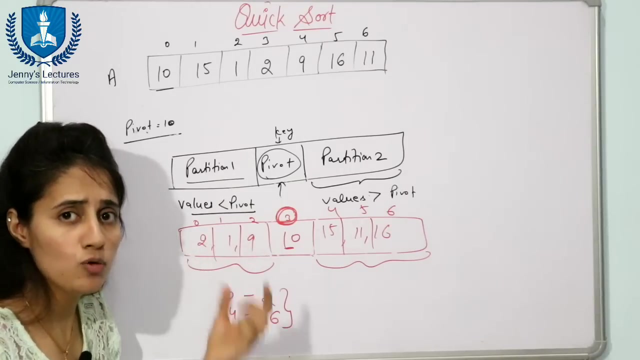 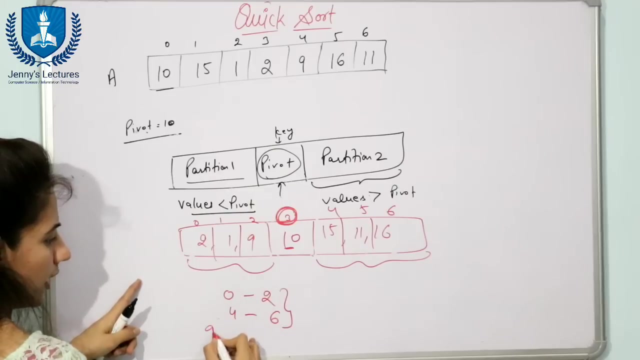 Because this is this. 10 is at its proper place now. Fine, Now see this. these elements are less than 10, but these elements are not in sorted order. So then you can say: these elements can be arranged in many ways. Maybe you apply some logic and you got that. to the left of this 10 you have 9, 2 and 1.. 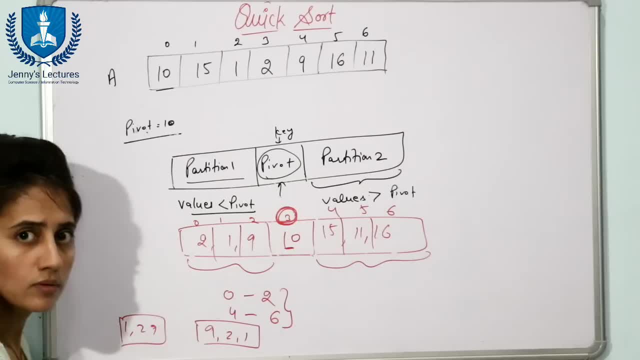 Or you have 1, 2 and 9.. Or you have 2, 1 and 9. So these elements can be arranged in many ways. It's not like that you will always got 2, 1 and 9.. 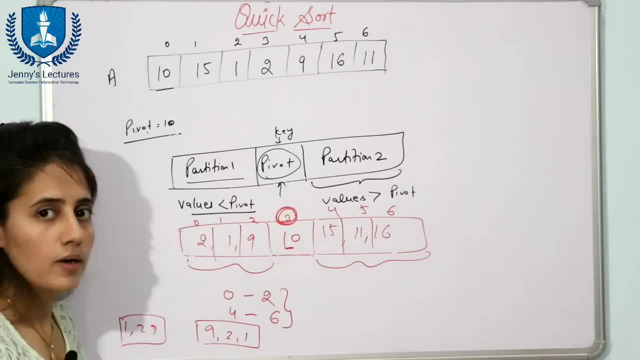 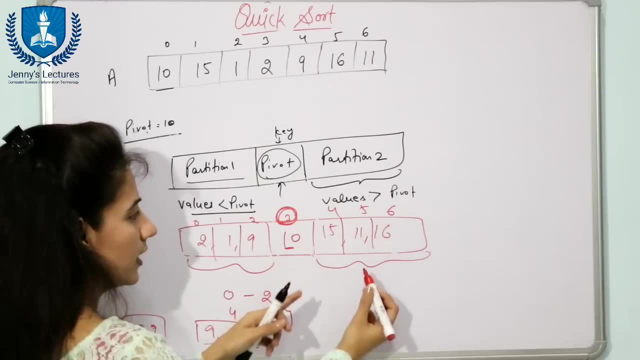 It depends how you are going to implement that partition logic And in the same way to the right also. Maybe I am getting the arrangement 15, 11 and 16.. Maybe you are getting the arrangement 16, 15 and 11.. 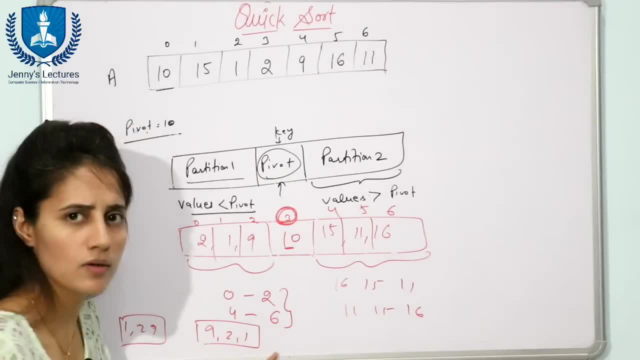 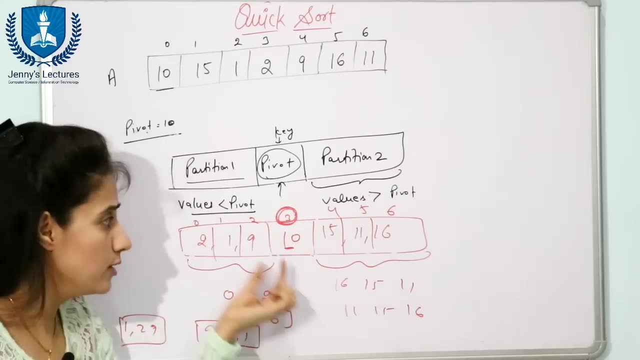 Maybe another one is getting the arrangement: 11, 15 and 16.. Like this. Okay, But that is for sure. all the elements to the right of this 10 would be greater than 10.. All the elements to the left of this 10 would be less than this 10.. 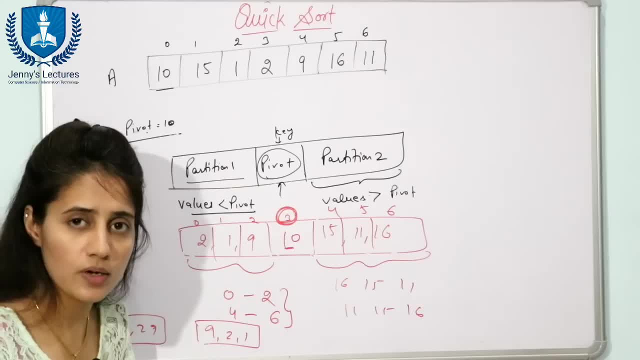 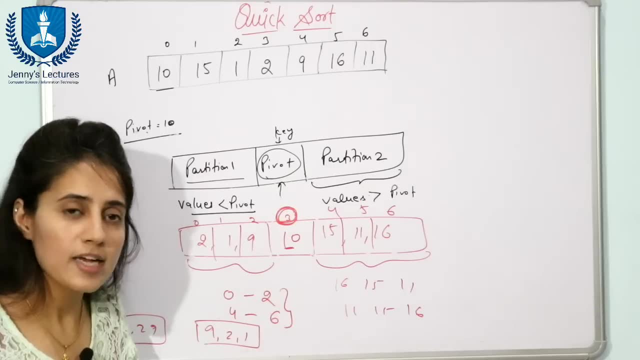 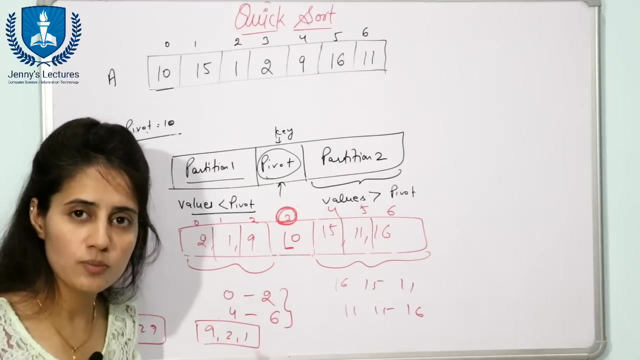 And same element or equal element can go either way. Fine, So this is the main funda. This is known as partition: Finding out the proper place for pivot element and partitioning the array into two parts. Okay, That is known as partition method. 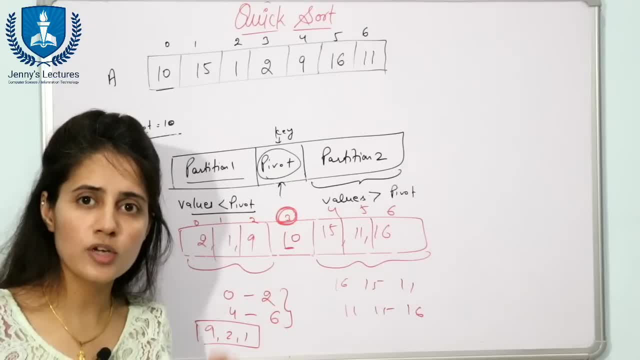 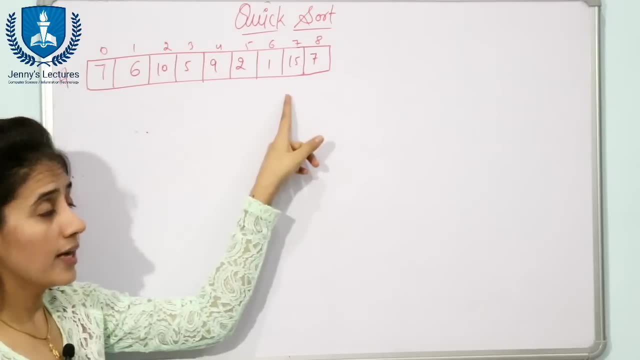 And this is the backbone of this quick sort. Now we are going to take one example and we are going to apply that quick sort on that example. So now let us take this example where we are having 9 elements in an array, Name of the array is a and index is from 0 to 8.. 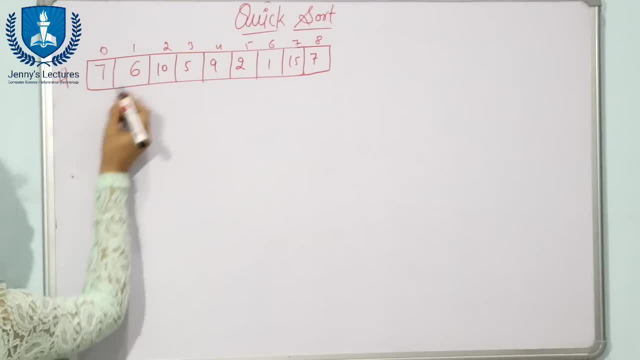 Okay, Now we are going to consider this, This element, This element, as pivot element. So pivot element is 7.. Or you can say, pivot element is a of this: 0.. Fine, So this is, you can say that lower bound of this array. 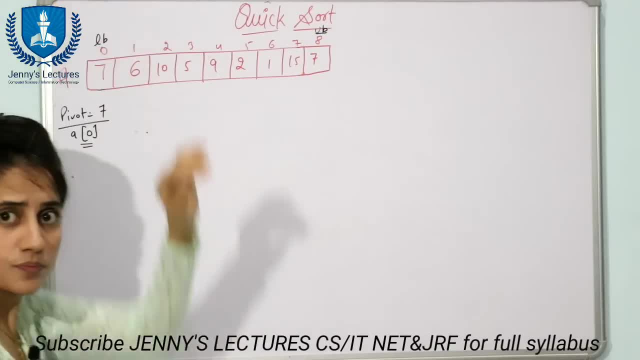 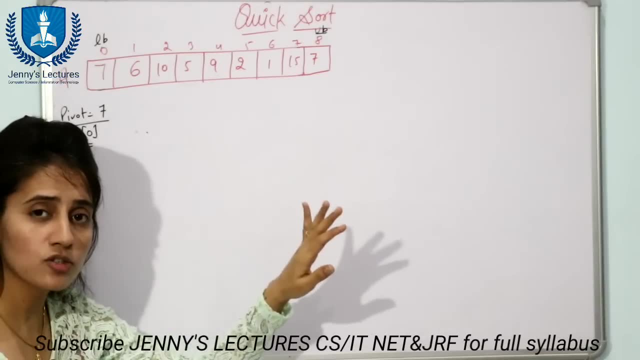 And this is what, upper bound, we have. Okay, Now, simple thing is you have to find out proper place for this pivot elements, such that all the elements less than the 7 would be to the left side, All the elements Greater than 7.. 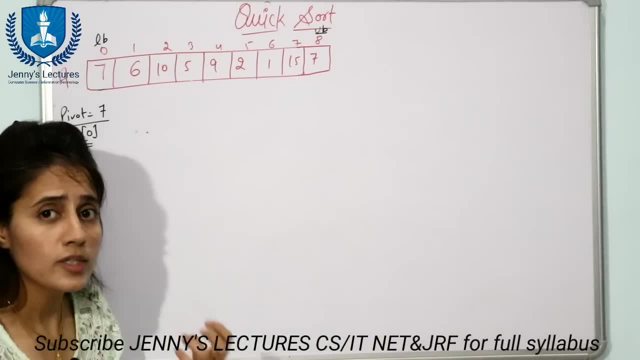 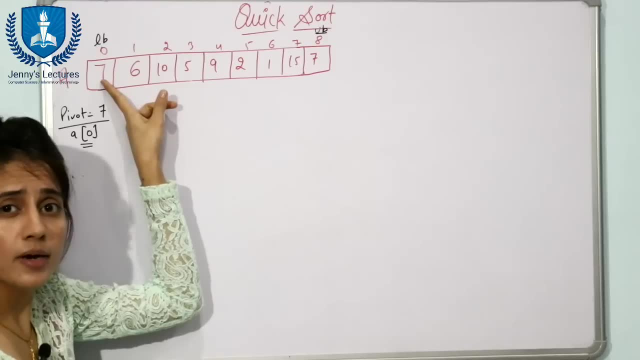 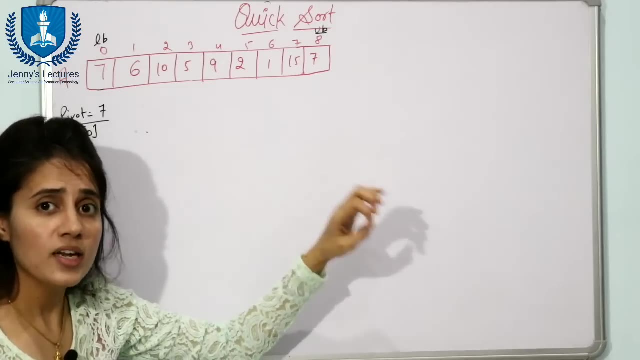 to the right side. So now what you are going to do is you can say that if any element is this side and which is greater than this pivot element, then we are going to move that element to right side. fine, to the right most right, most side, you can say: and if any, any element is this side, 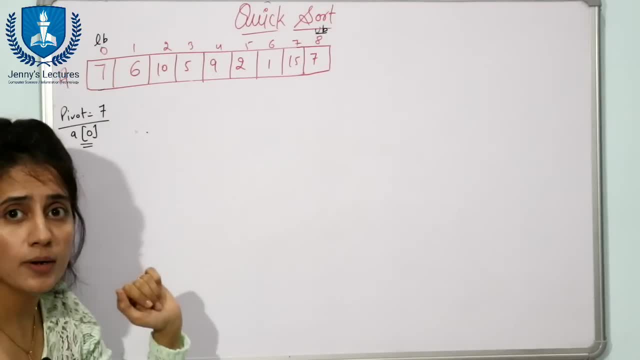 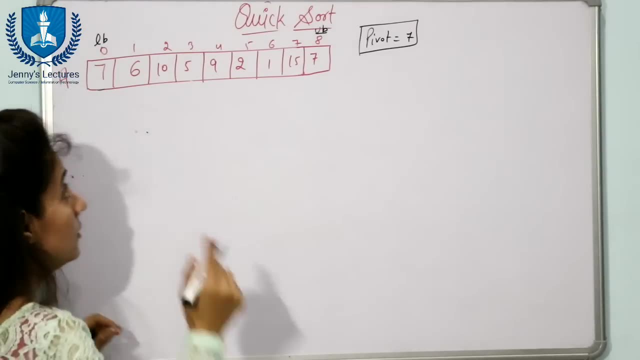 and if that element is less than this pivot element, then we are going to bring that element to this side. so i am going to take now two variables. one is suppose here we have start and here we have end. okay, i am going to move the start from this side to this side and i am going 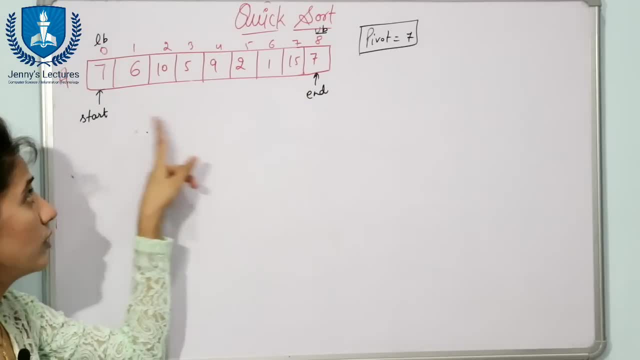 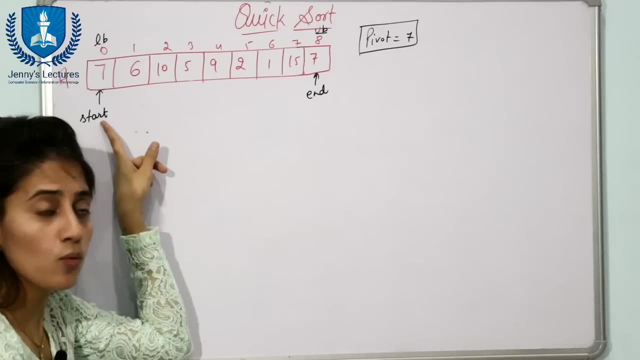 to move this end from this side to this side, right to left, and this to left, left to right. if we are going to move the start from left to right, then obviously we are going to increase this start. we are going to increment this by one: first of all zero, then one, two, three, like this: 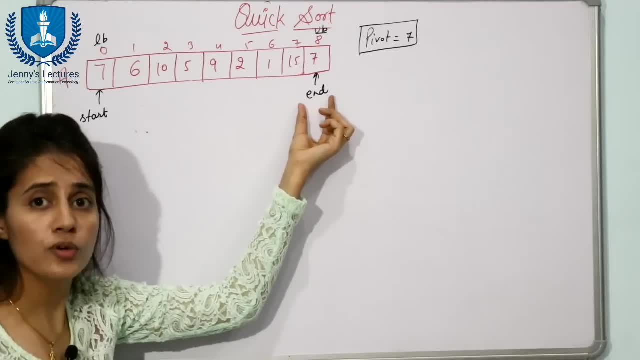 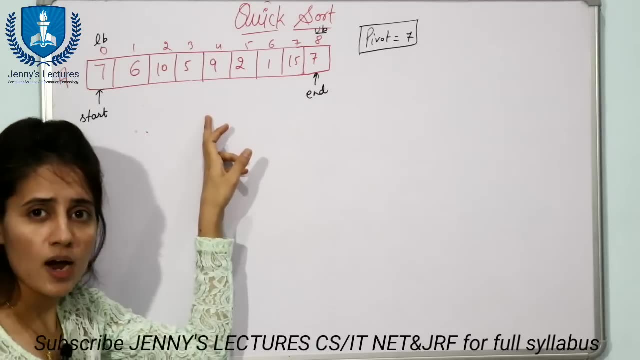 and if you are going to move this end from right to left, then we are going to decrement this end, that is for sure. okay now, what are the conditions? if you are incrementing this start? when you are going to stop this, if you are decrementing this, end when you are going to stop this. 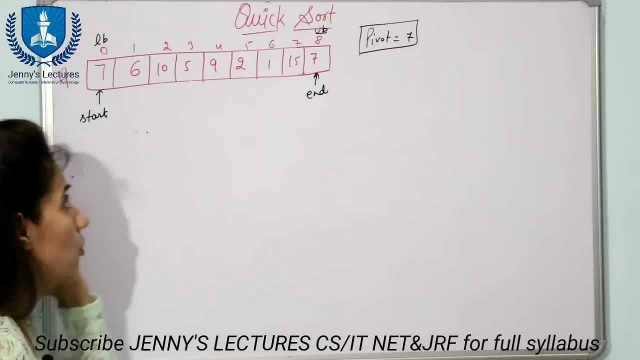 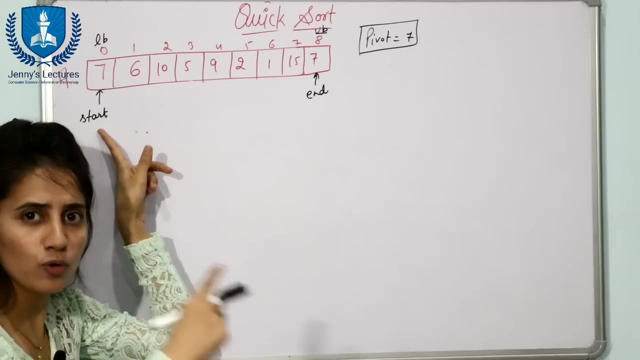 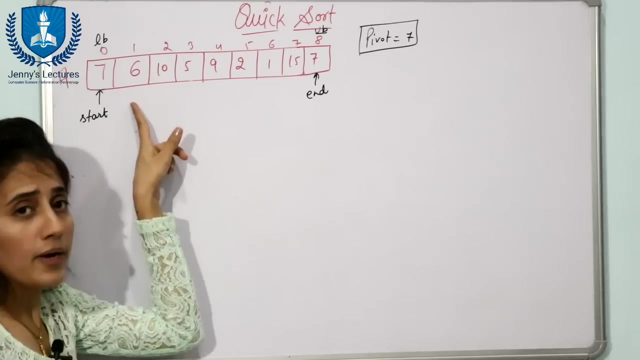 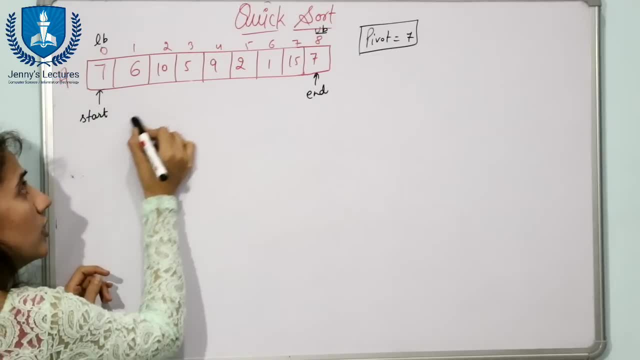 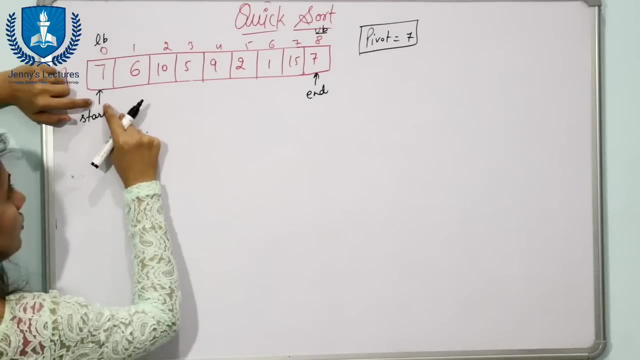 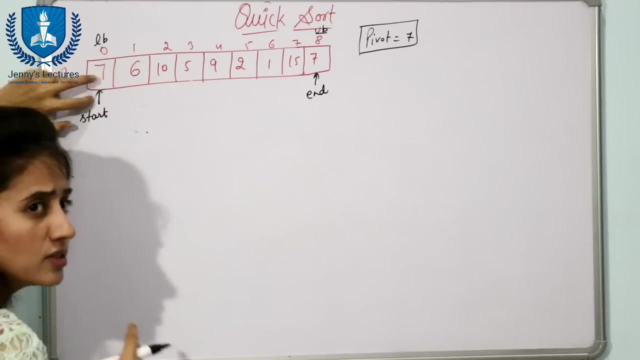 or equal to this pivot element, then we are going to increment this until we found element greater than pivot element. see now. see, start is at this place. first of all. now, pivot element is also this and start is also this: now the seven is less than or equal to: 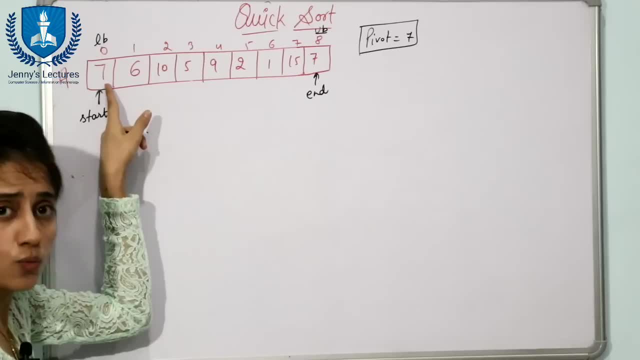 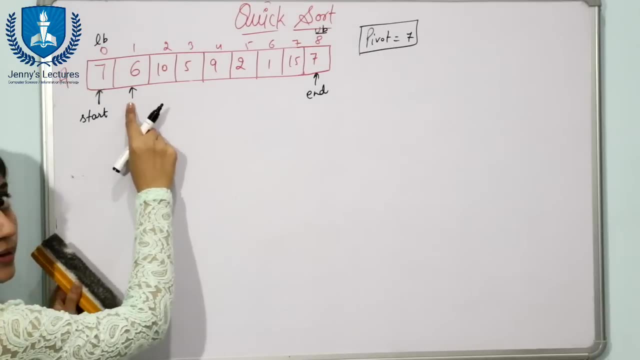 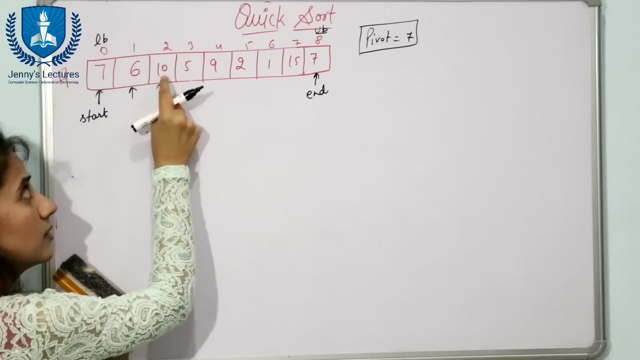 pivot element. yes, because it it is equal to this pivot element. then we are going to increment this. start now. start is at this place. fine, now six. six is less than pivot element. yes. again, increment start. 10 is 10 less than or equal to pivot element no. 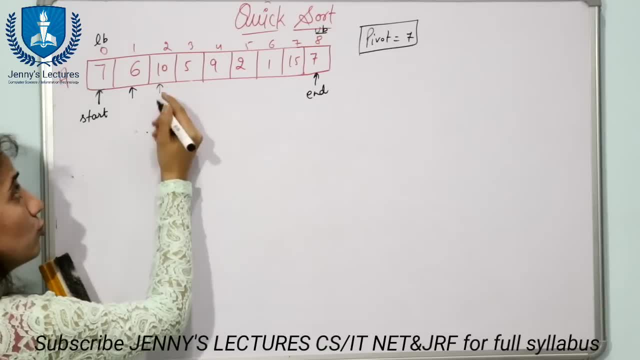 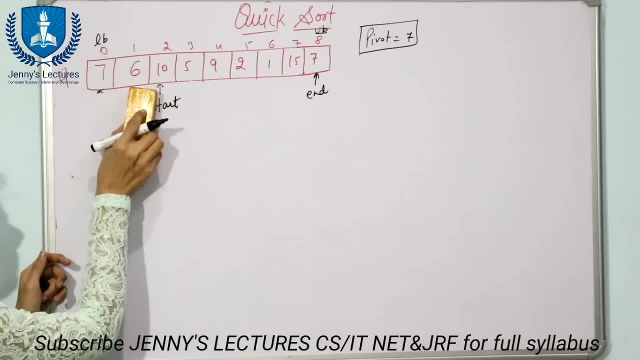 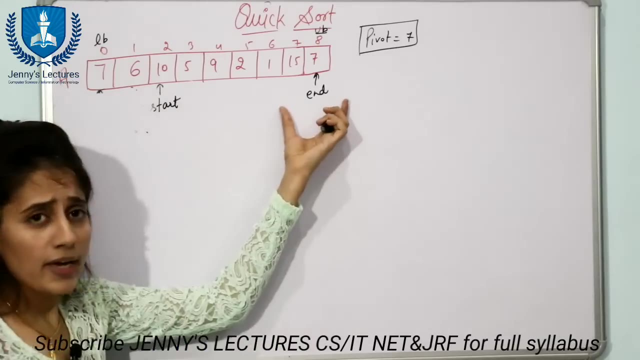 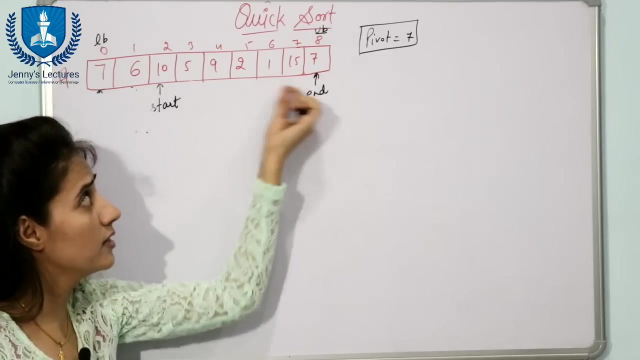 we found greater element than pivot element, then we are going to stop here. now start is at this place. fine, now end. what about this end variable? from here we are going to find out what an element which is less than pivot element, if element is less than pivot element and which is at this side. 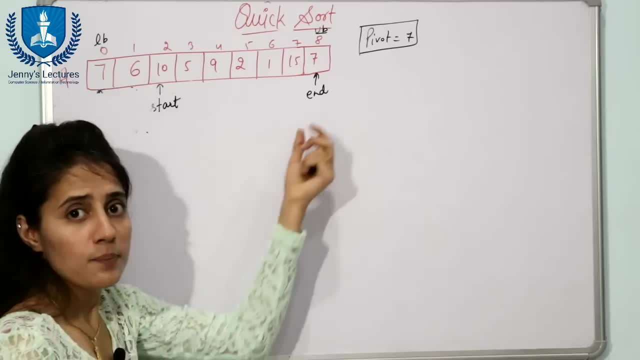 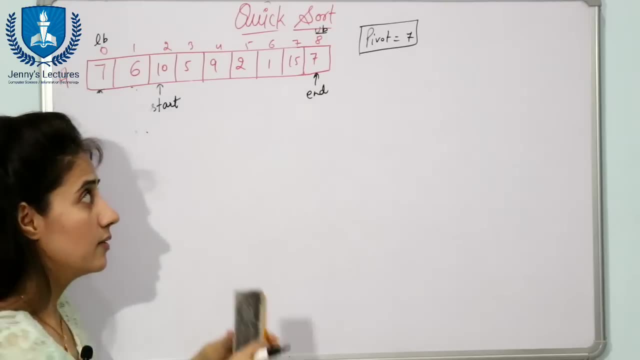 then we are going to move that element to this side. or in simple terms, you can say: it is less than pivot element. guess what if you, if you are finding an element which is greater than greater than this pivot element, then you are going to decrement this until you find an element which is less than pivot element. 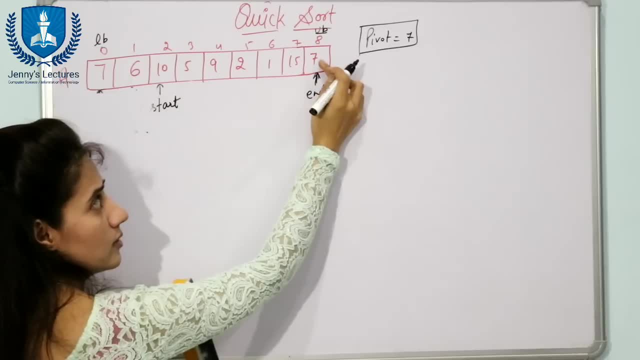 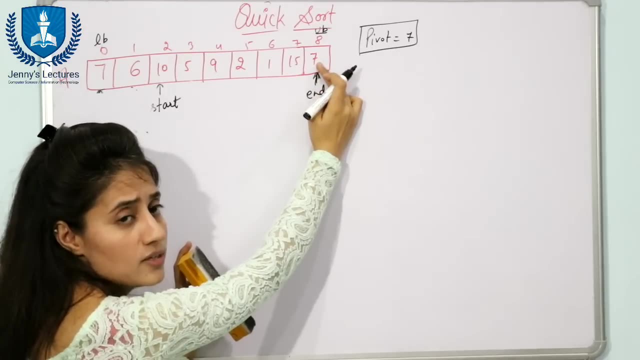 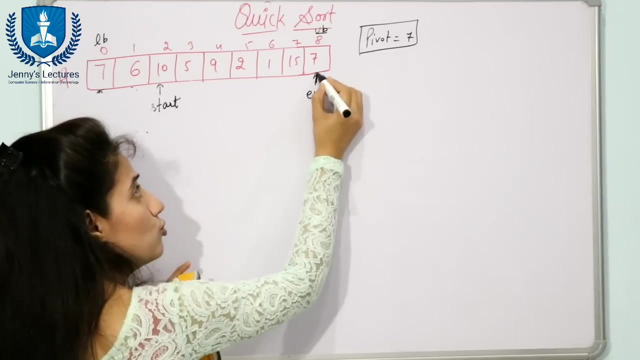 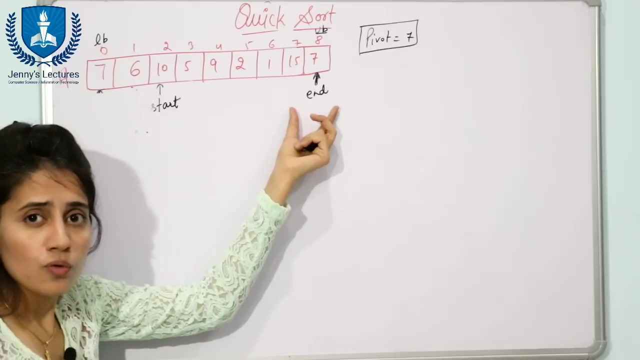 now see. start at starting end is at this point: 7 is 7 greater than this pivot element. no 7 is equal to pivot element. fine, greater than it is not greater than this pivot element, then we are going to stop here. only we are not going to decrement this end. fine, now what you will do. you. 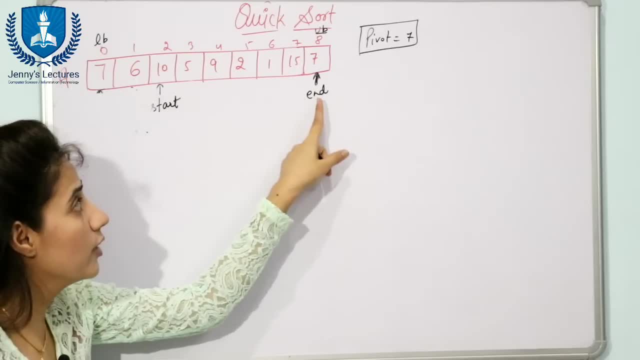 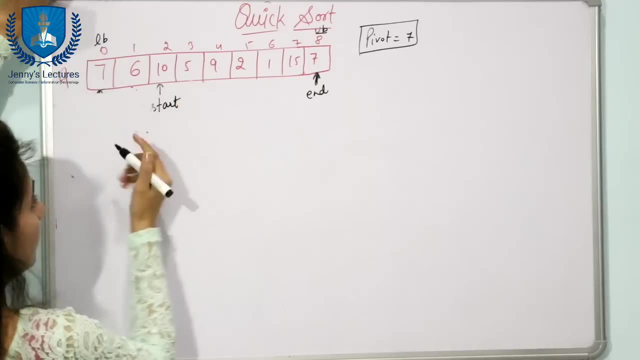 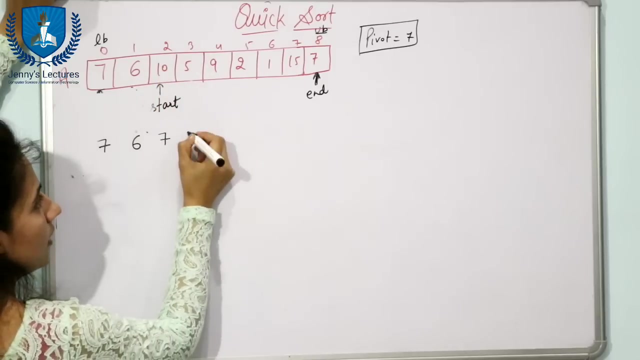 now you are going to swap this, a of start with a of end, these two values. now, after swapping what? what would be the day? what would be the array? here we have seven, here we have six. the seven would be swapped with this ten. here we got seven, again, here we got five, nine, two, one, fifteen and 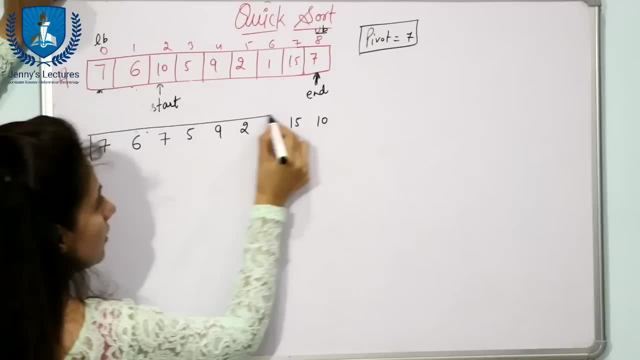 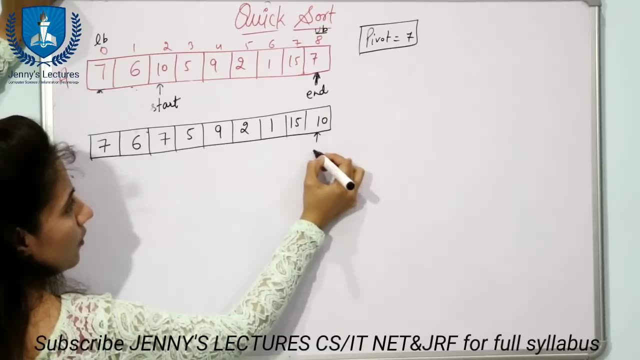 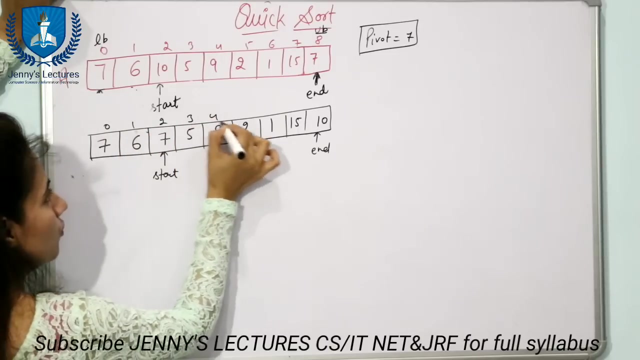 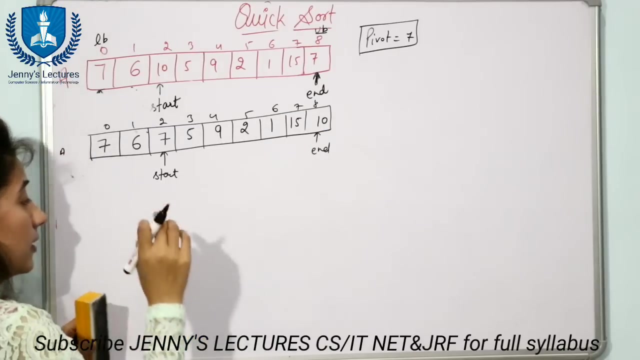 ten would go there. now, this is our array after first swap. fine, here we have end operator and here we have start zero. one, two, three, four, five, six, seven and eight. this is a. now again check a of start. a of start is seven. seven is less than eight. 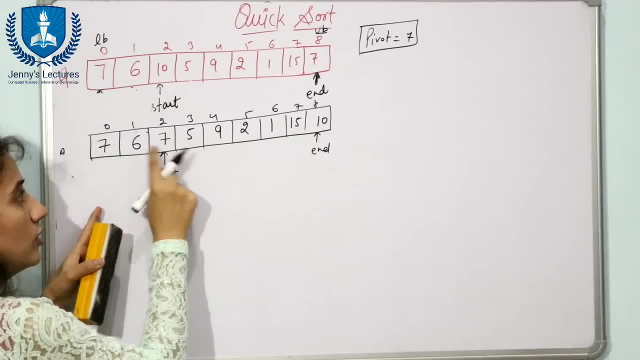 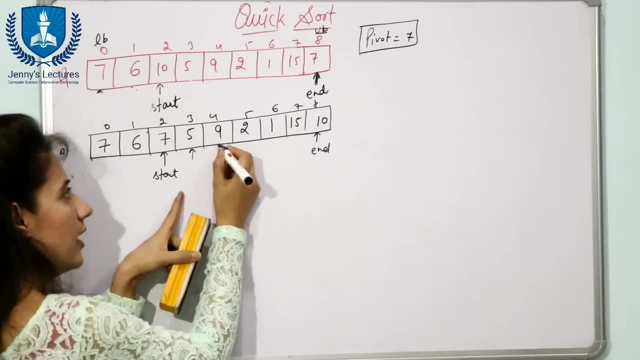 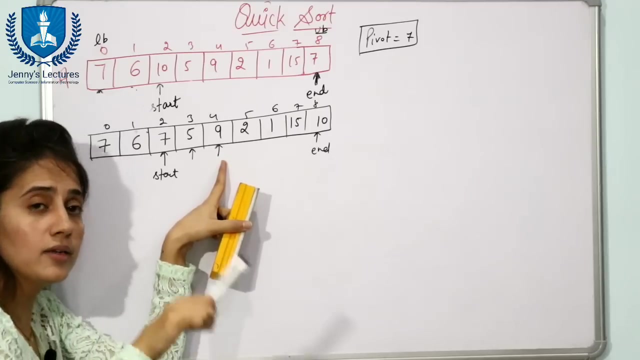 then equal to pivot element. yes, seven is equal to the seven. then we are going to increment this: five is less than pivot element. yes, again, increment nine less than equal to seven. no, we got greater element than this pivot element. then we are going to stop here. now start is at this position. 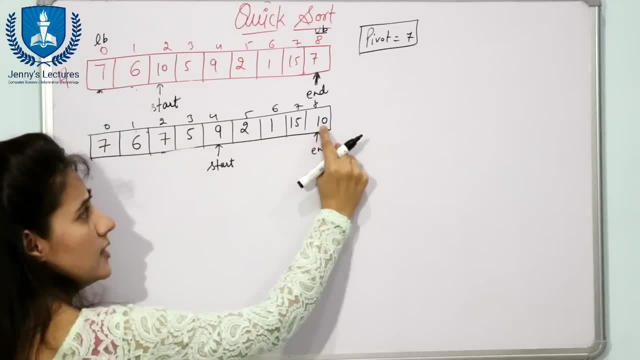 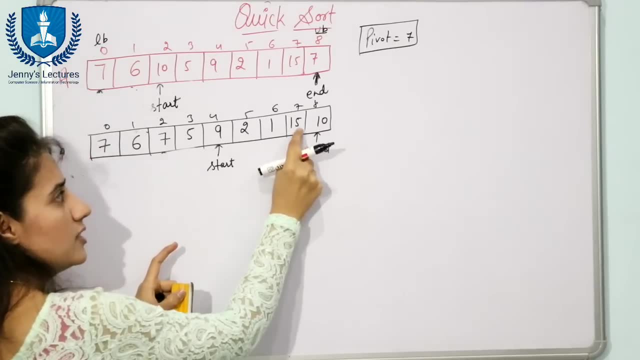 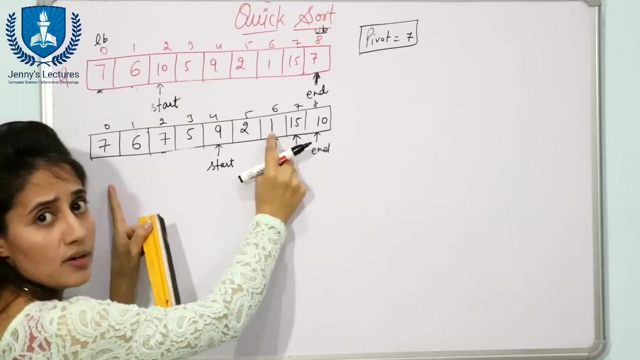 now for end check a of end. is this element greater than this pivot element? pivot is seven. yes, we are going to decrement this element. 15 greater than 7. yes, we are going to decrement this is 1 greater than 7. no, we found an element. 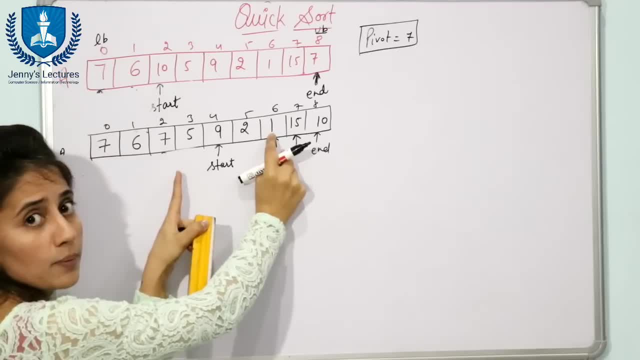 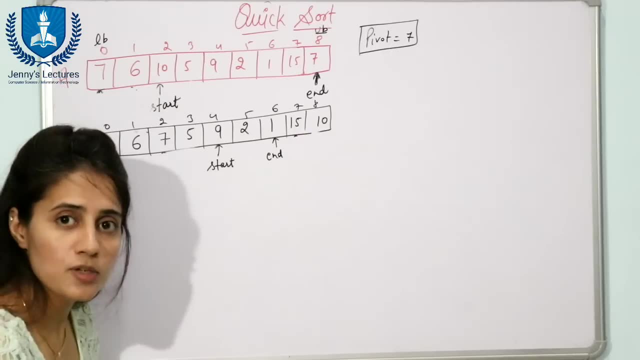 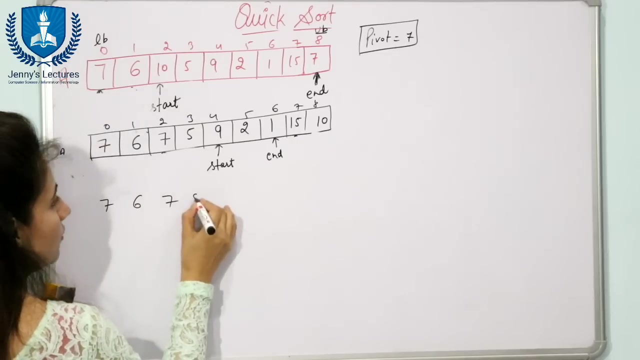 which is less than which is less than pivot element, then we are going to stop here now and is at this place. next step is what you are going to swap this with this. fine, after swapping, the array would be seven, six, seven, five, nine. sorry, here we have one, here we have two. here we. 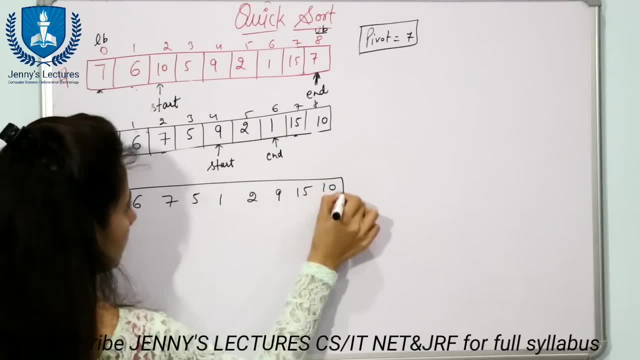 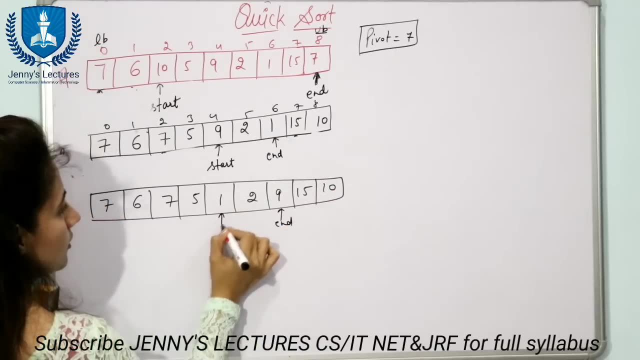 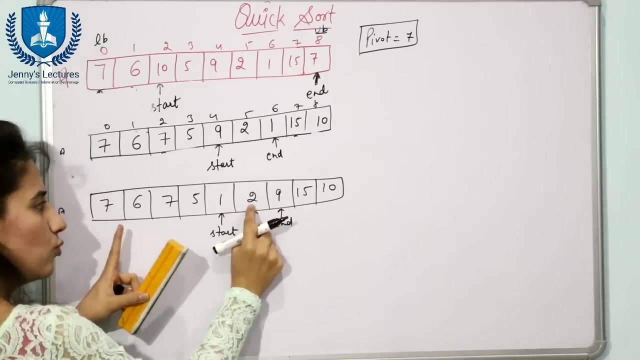 have 9, 15 and 10.. okay, and start end pointer is here only and start pointer is here only. fine, again. apply same funda a of start check: less than equal to pivot element: Yes. Increment start: Less than equal to pivot element: Yes. Increment start Is this: 9 less. 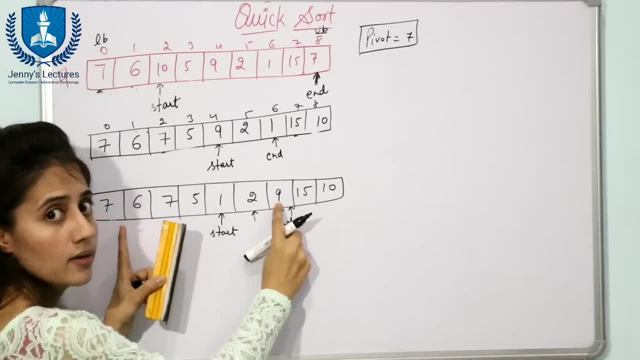 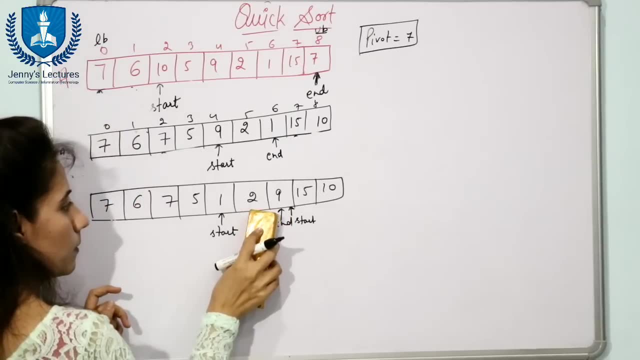 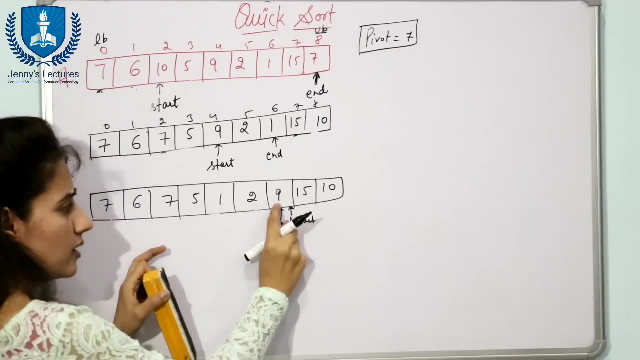 than or equal to pivot element. No, It is greater than. So we are going to stop here now. Now, at start, is at this position For end Check, Because we are going to decrement this end. A of end is 9.. Is this greater than pivot element? Yes, Then decrement. 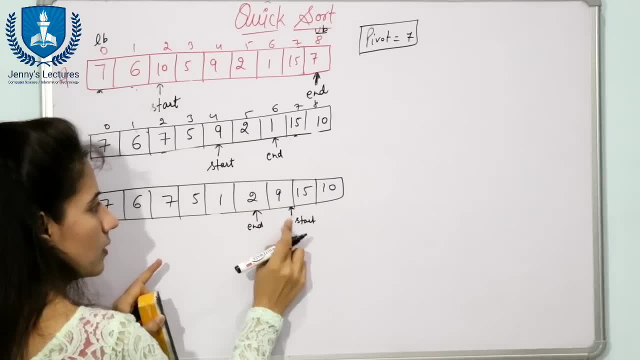 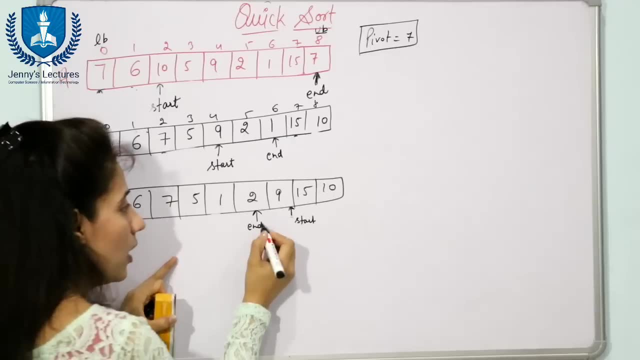 Now end is at this place. 2. Is 2 greater than pivot element? Pivot is 7.. No, Then we are going to stop here. only Now end is at this place, But after that step is what We are going to swap. 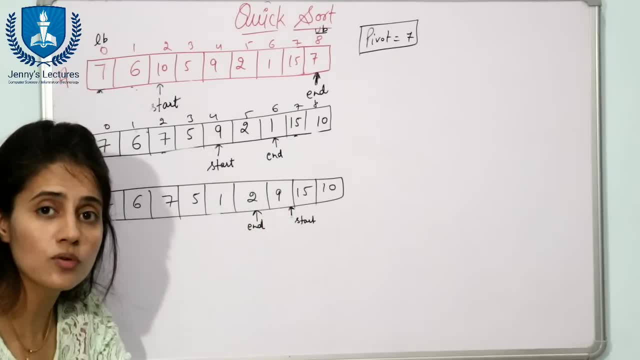 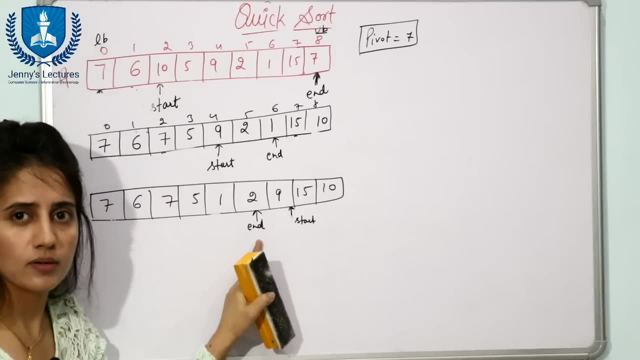 these elements. But here we are not going to swap these elements. Why so? Why so? Because this start variable has crossed end variable. Okay, Start is now greater than end, So now we are not going to swap these elements. Fine, If start is, we are going to follow the procedure. 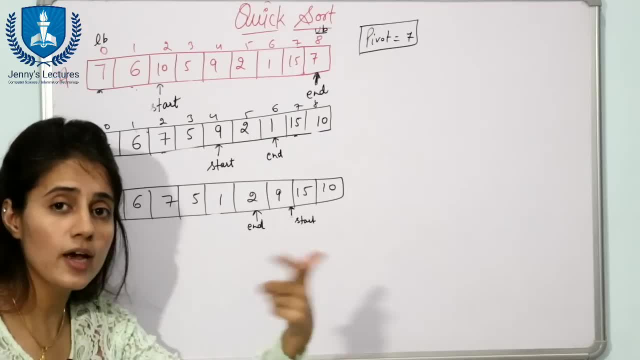 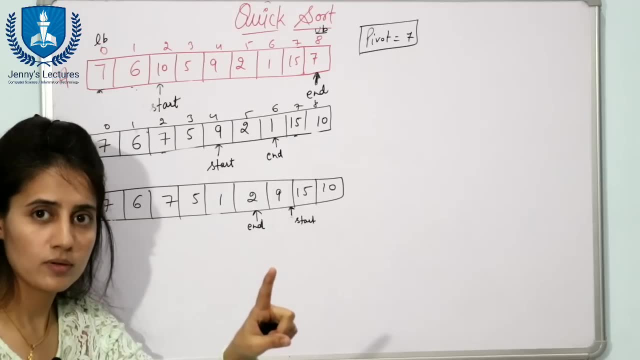 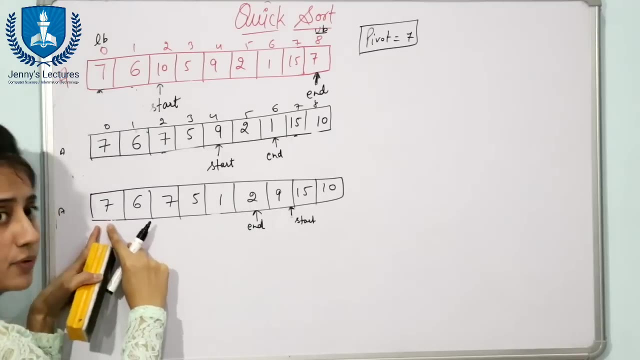 of swapping, and all until we till we have start is less than end. At the point we got start is greater than end, then we are not going to swap. Fine, Now. next Step is what? Now we are going to swap what? this pivot element with this element, The element, 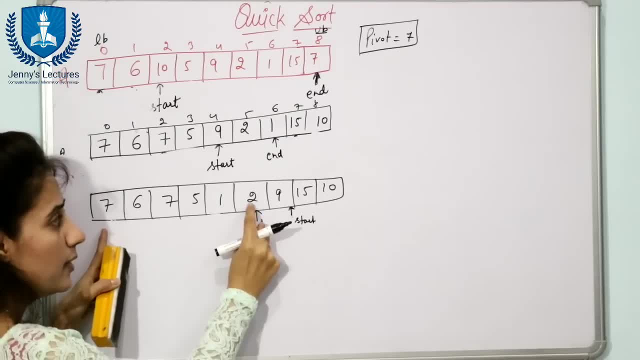 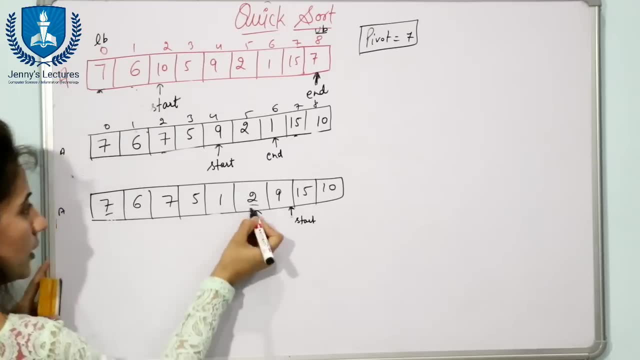 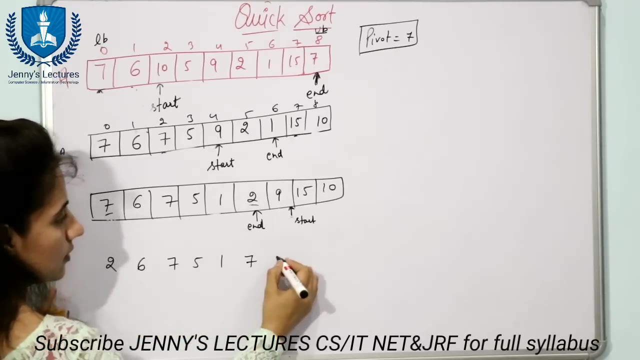 which is at this position. At this position, element is 2.. Pivot element is what? 7.. Now we are going to swap these elements. So, after swapping, array would be 2 would go here. Now, here we have 6,, 7,, 5,, 1, and here we have 7,, 9,, 15 and 10.. 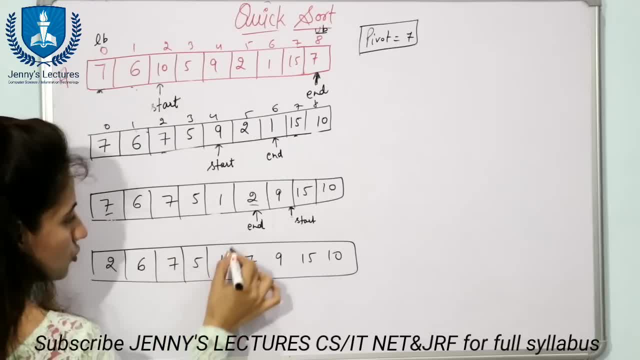 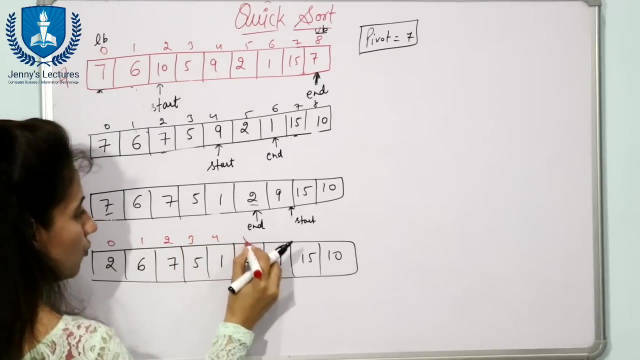 So this is now the array. Now see, this was the pivot element and we got this element here only. Fine, And 0,, 1,, 2,, 3,, 4,, 5,, 6,, 7,, 8, and the location for this is 5.. So now you. 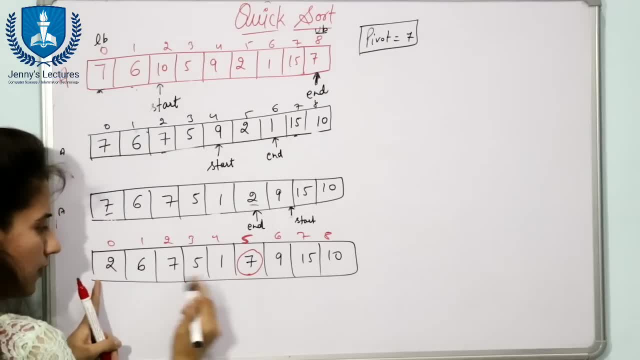 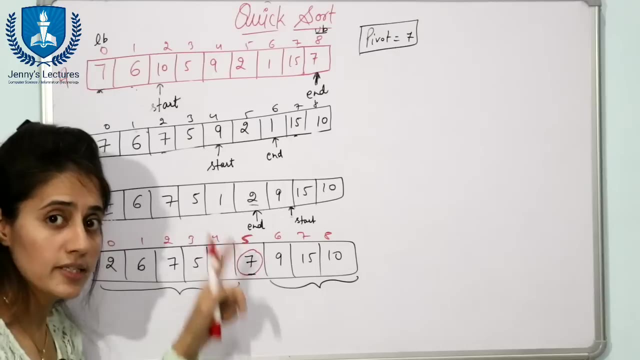 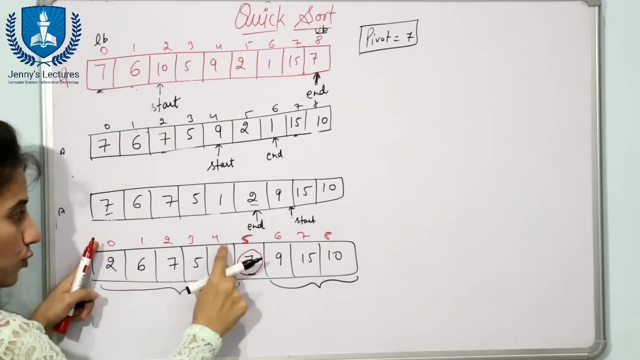 can check. all the elements which are less than or equal to this 7 are to the left of this side. Now, this is at its appropriate place. Now you are going to apply the same funda on this partition, and on this partition Till 0 to 4 and 6 to 8.. Same from this partition, you are. 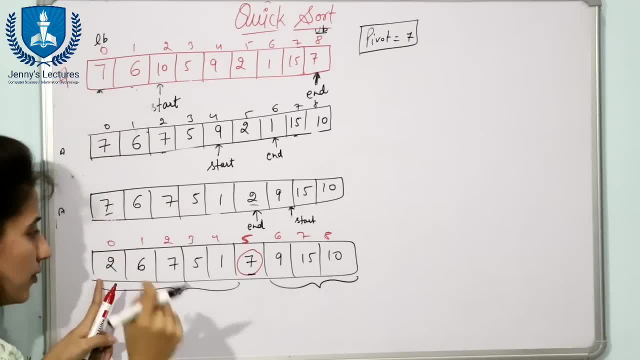 going to choose pivot element, Starting element. we are going to choose pivot element So 2. we are going to choose as pivot element Fine And rel variables would also be there. only Start element would be there. To variable would be there. Start from here and end from. 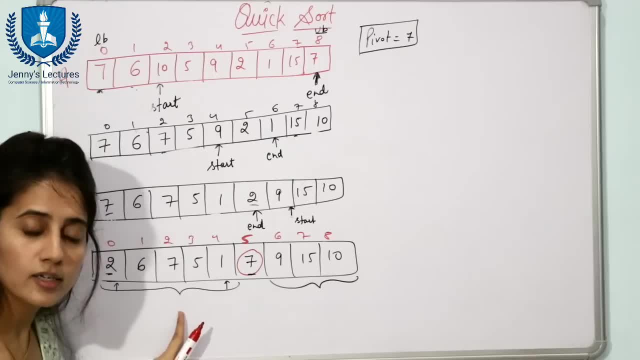 here only, We will increment this start till we find and element which is greater than than this pivot element, And we are going to decrement this end till and until we find an element which is less than the pivot element, and then we are going to swap these elements. 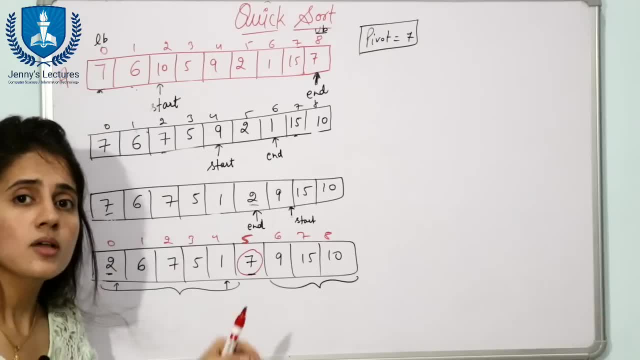 or you can say exchange those elements. that is why it is also known as partition exchange sort. Fine, Now, this is finished. Now is that I want to? I want to correct by git disk space h1 to git and gits Ntr. and when we enter into view input ntc, where we will go to these variables, we can see that now is dumpling. uh, vaakpa surface is now there anymore. So let's see the last step here Here, jrica one, can we kind of 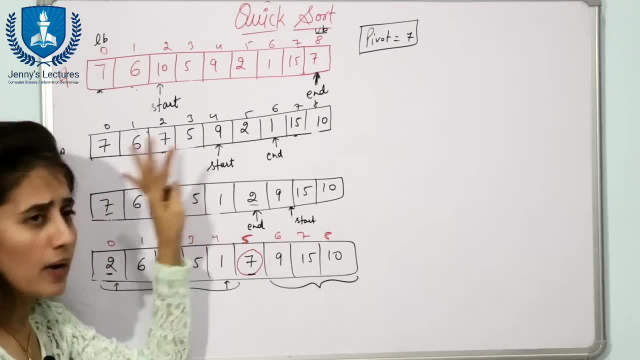 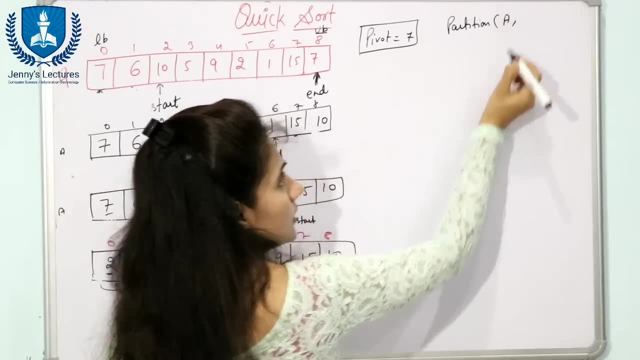 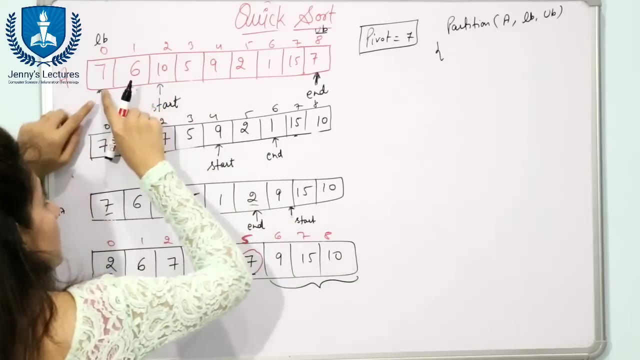 fine now if if i write down this partition method into coding, then how we will write. we have one function that is partition. we are going to pass a is name of array, lower bound and upper bound. right after that, we have chosen one element, starting element, as pivot element, so we 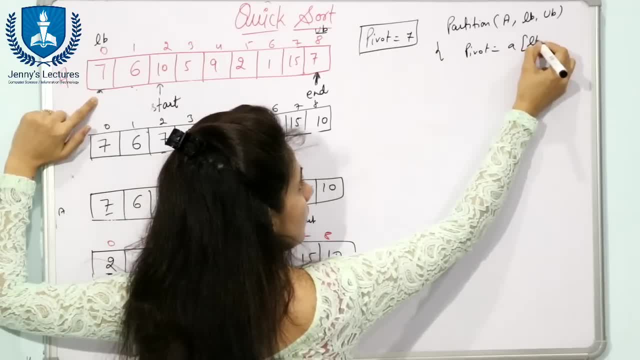 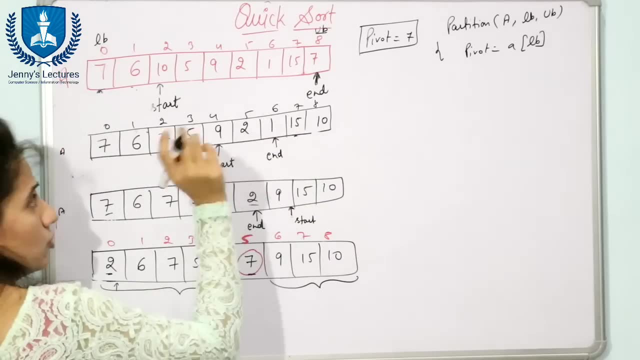 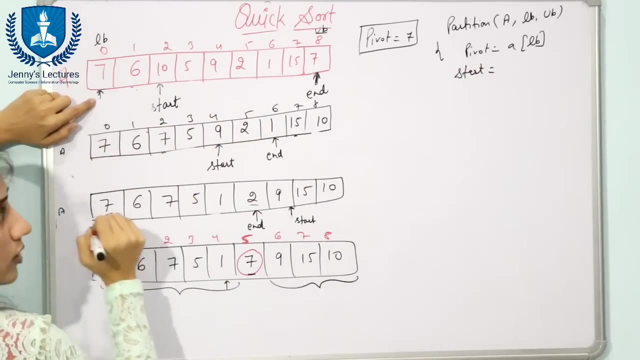 will write what pivot is equal to a of lower bound, because lower bound is 0 and upper bound is this: 8, okay, next, we have taken two loops, sorry, two variables, start and end, and we have initialized start. from here only you can say: start is equal to lower bound and end is equal to upper bound. 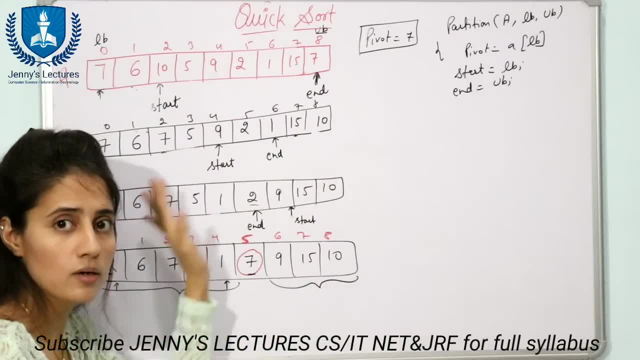 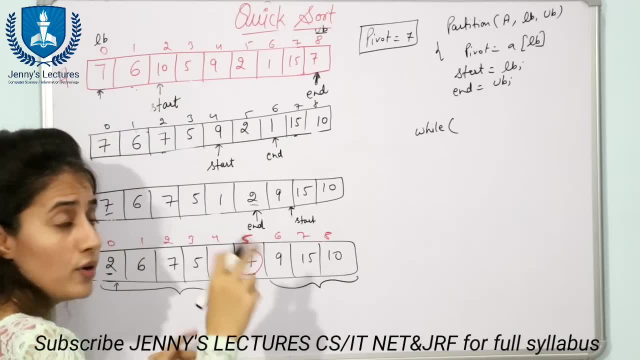 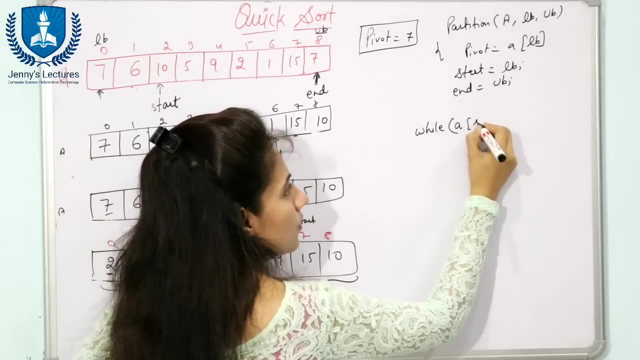 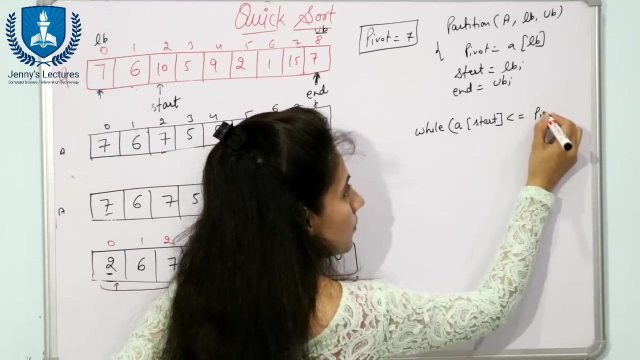 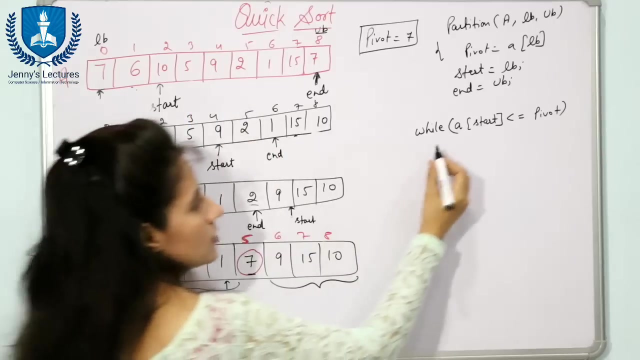 and was at this place. now we are going to apply the loop, see, while we have incremented this start. so what we have checked: while a of start is less than less than equal to pivot, if a of start is less than pivot, then we are going to increment this start. then we are going to do what start. 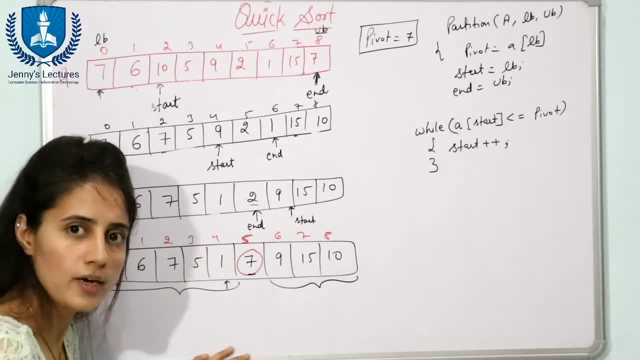 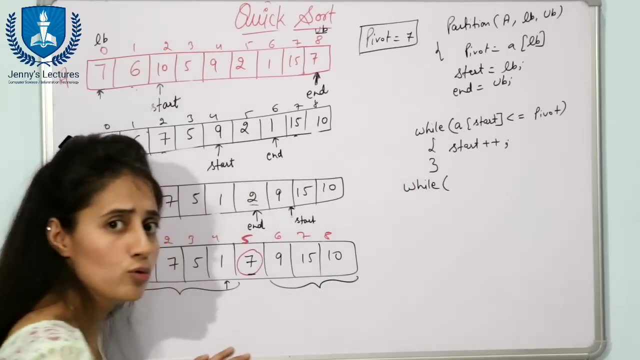 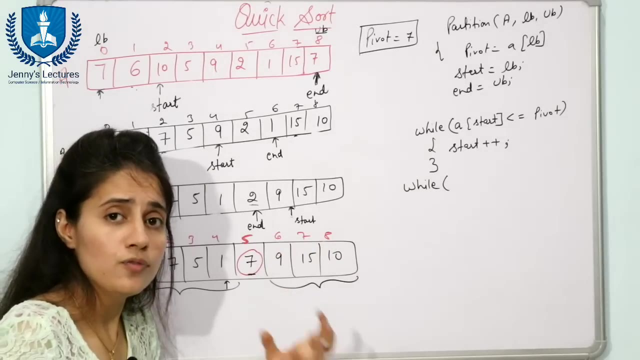 plus, plus, right and next was decrementing of this end. and when you will decrement this? when you are going to stop this. if you find any element which is less than pivot, then you are going to step. stop this if you find, if you find element which are greater than pivot, then you are going to 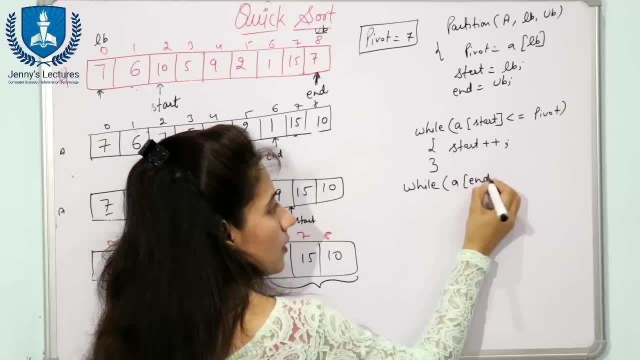 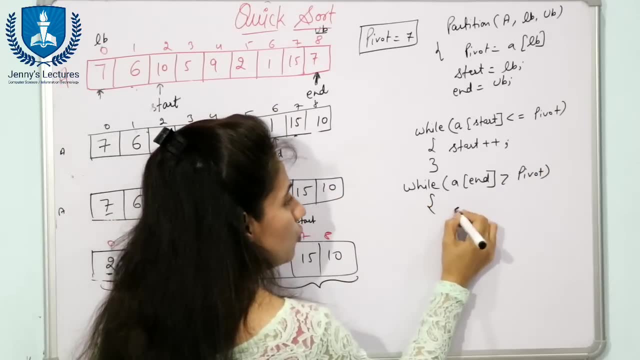 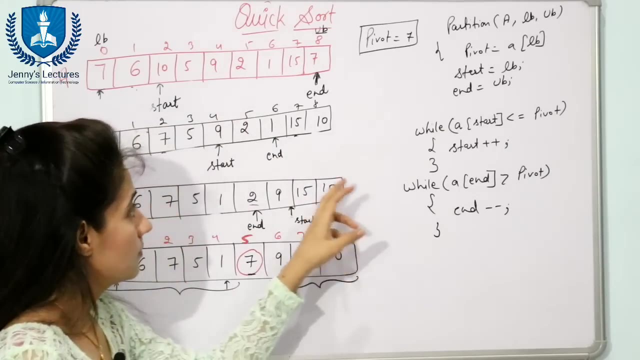 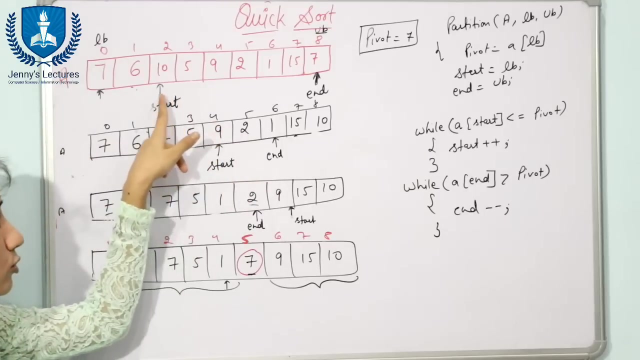 decrement, end. so while a of end is greater than a of start, pivot element, then what you will do, end minus minus right. and if this condition is not true, this condition is also not true, then what you have done, you have done what swapping of those elements here or here. also see here a of start, a of start 10. 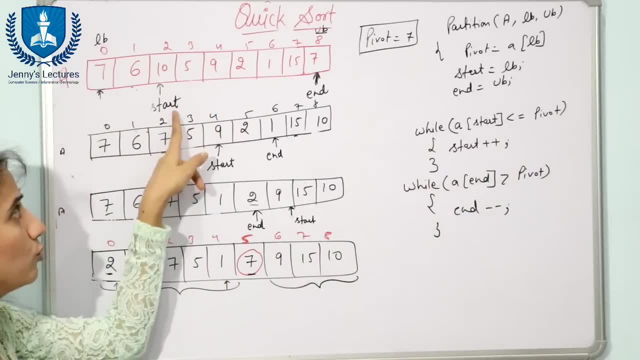 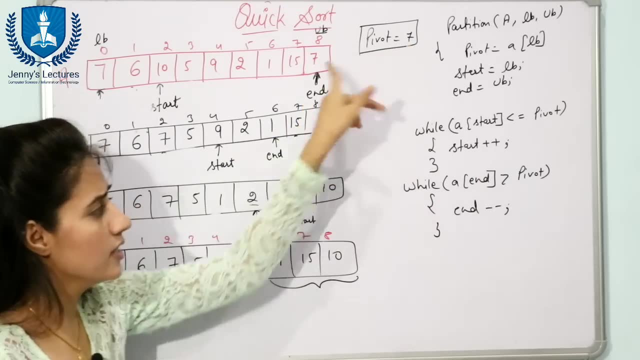 10 is less than equal to pivot. no, then, we are going to stop this. no, we are not going to increment this one a of end. a of end is 7. 7 is greater than pivot. 7 greater than 7. no, we are not going to do. and minus, minus. if this condition is not true, we are not going to do. and 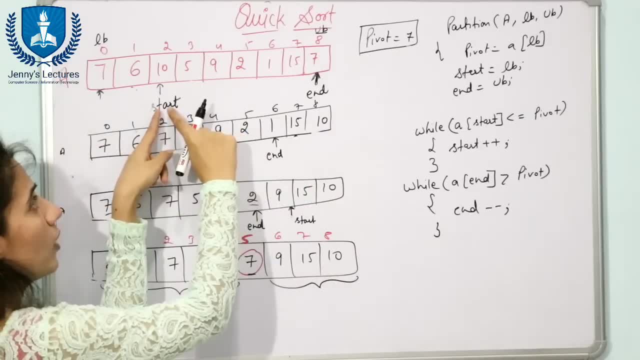 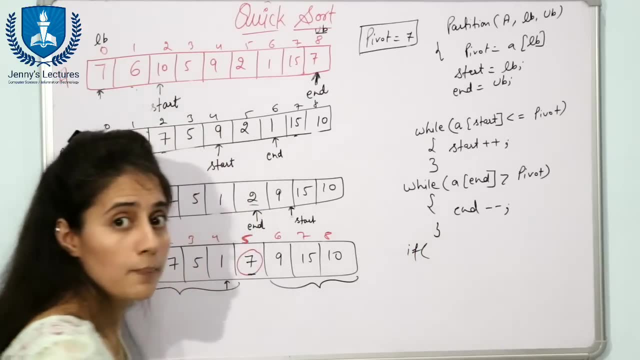 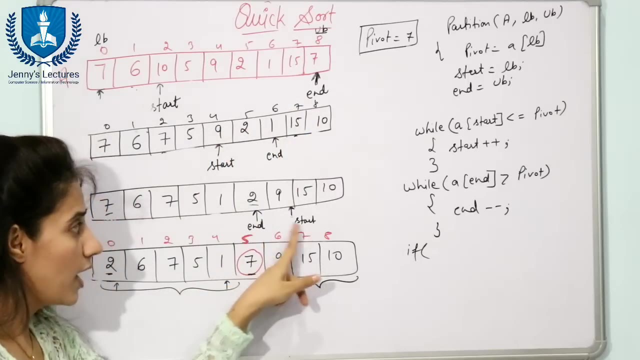 minus, minus. so we are going to stop here. after that, what we have done: we have swapped this with this, 7 with 10, right. so here what you will write. but if you do swapping only if this start is less than end. if you got start is greater than end, you are not going to swap. so you have to check one. 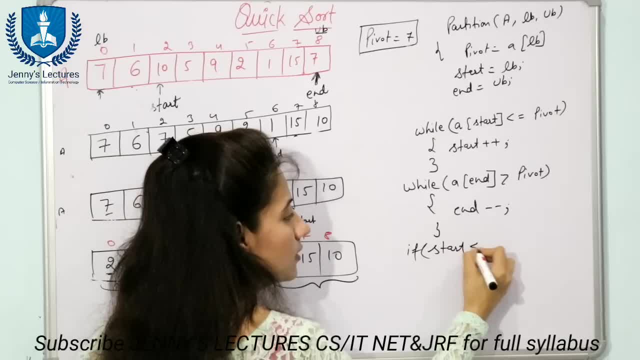 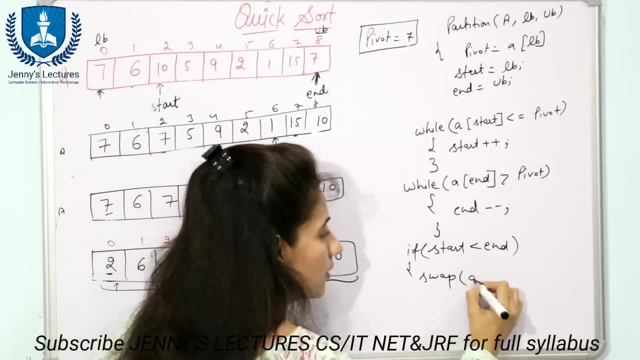 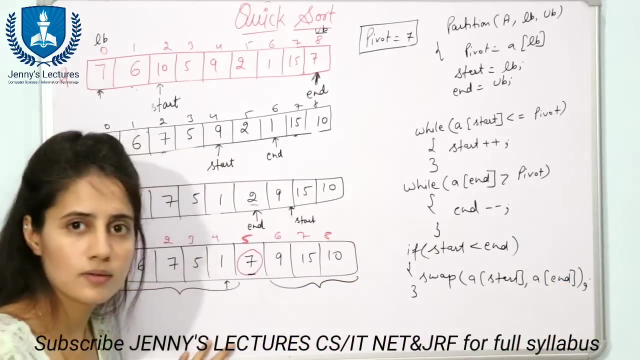 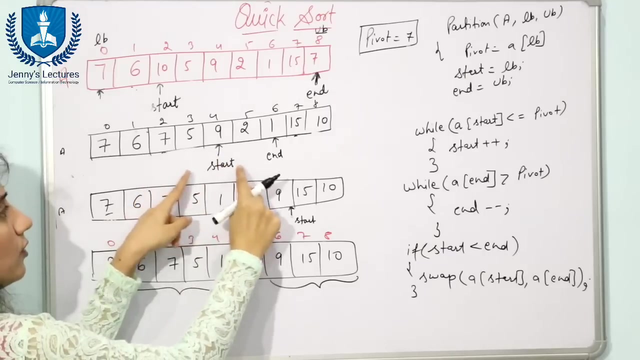 more condition before swapping: if start is less than end, then you are going to do what? swapping of a of start and a of end and you are going to repeat this process. see, here we have done swapping. after that, again we have checked start and end. again we have done swapping. again we have checked, but here we didn't. 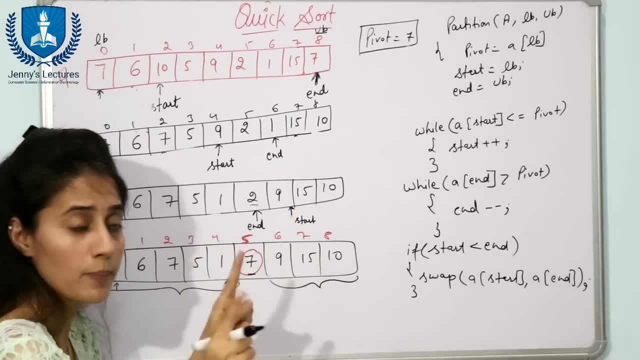 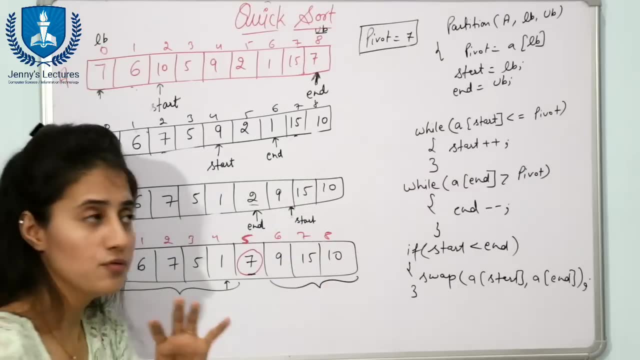 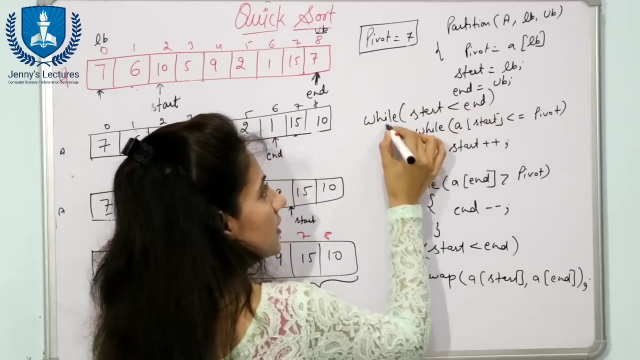 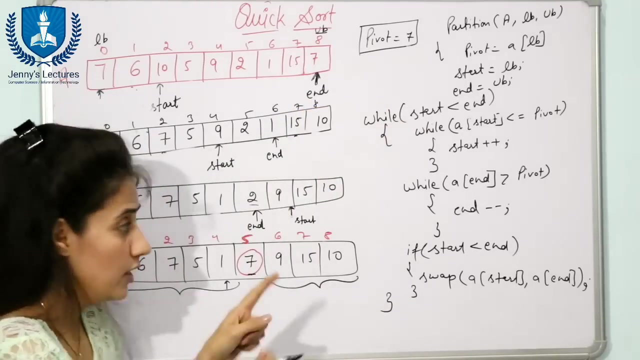 have swapping here. we didn't do any swapping because the start is greater than end, so you are going to follow this process if, or you can say, while while start is less than end, only in that case you are going to follow this process. if start is greater than end, in this case. 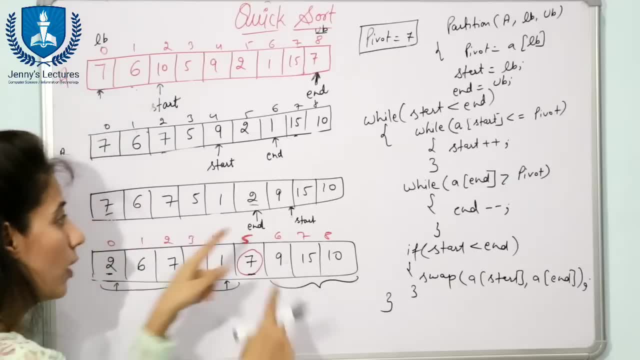 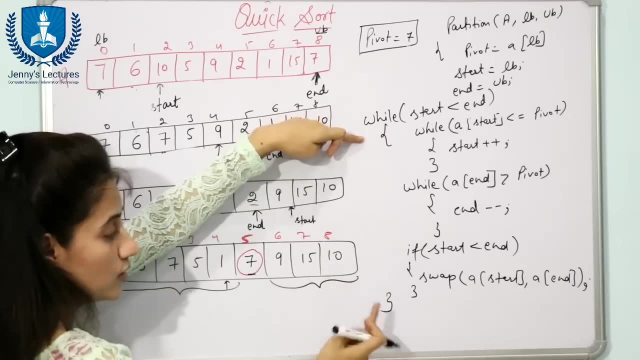 because start has crossed this end. in that case, what you have done? swapping of this and pivot element. so if this condition is not true- start is not less than end- then after that you will go out from this loop and after that what you will do? swapping, swapping of what swap. 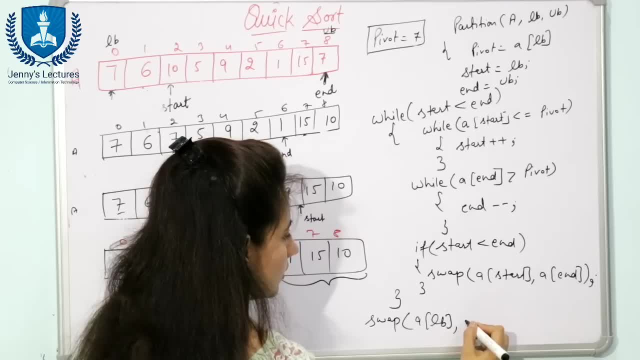 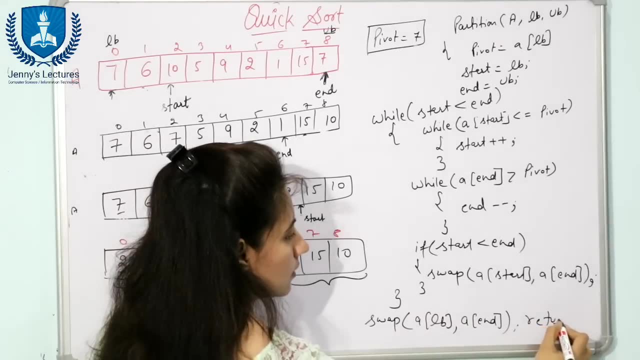 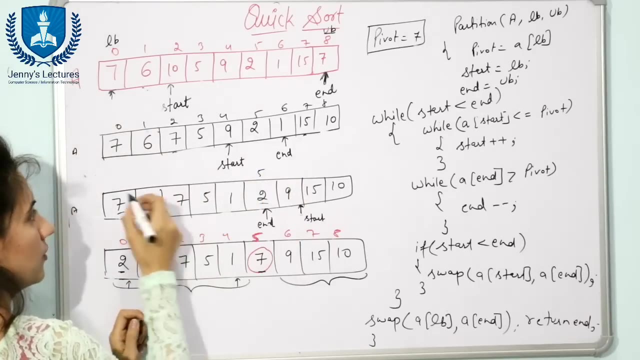 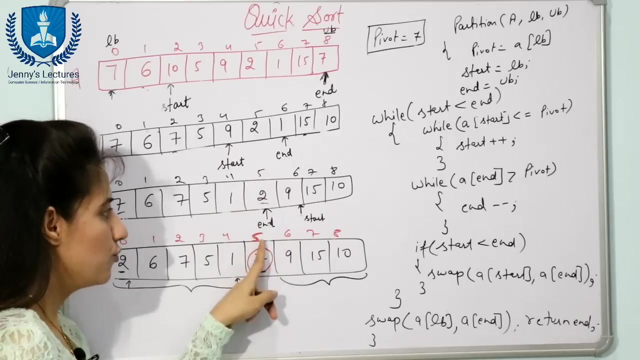 a of lower bound with a of end, and after that we will return what return? end, this end, this position, that is here we have index five, zero, one, two, three, four, five, six, seven, eight, eight. then we are going to return this and that is five, because after that you, you are going to apply. 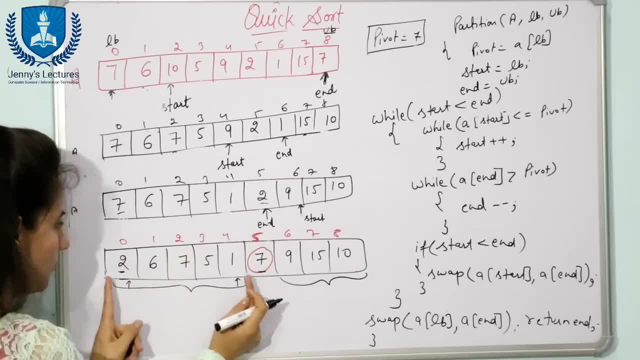 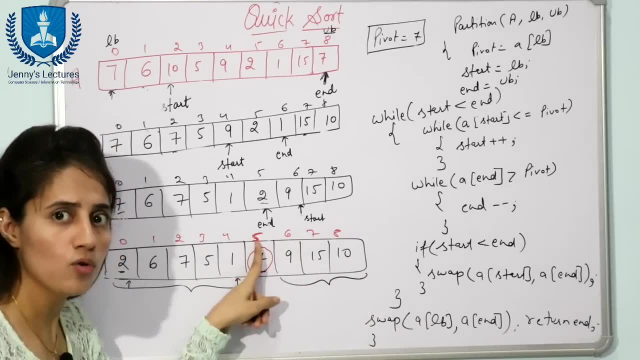 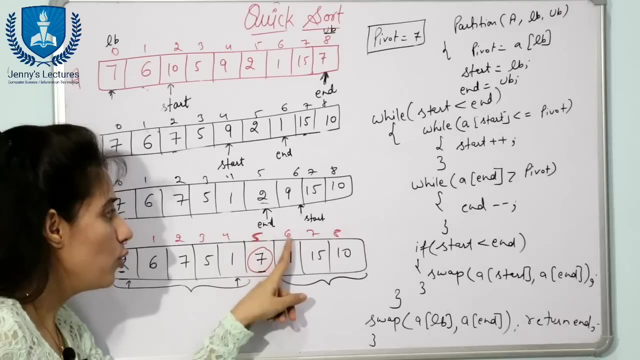 the this, this process, this partition process from zero to four and then from six to eight, and if you know this location, that that is five, then only you can say that we are going to apply from this lower bound to this location minus one and from location plus one to upper bound. that is where we are going. 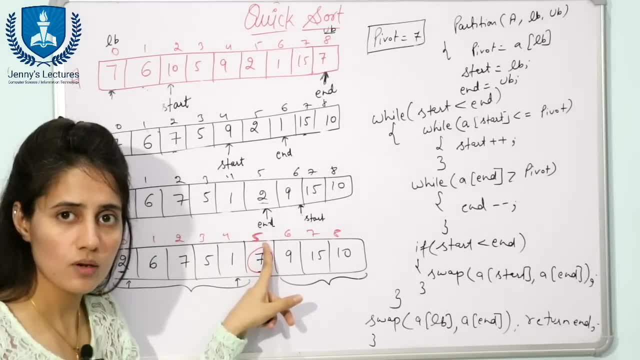 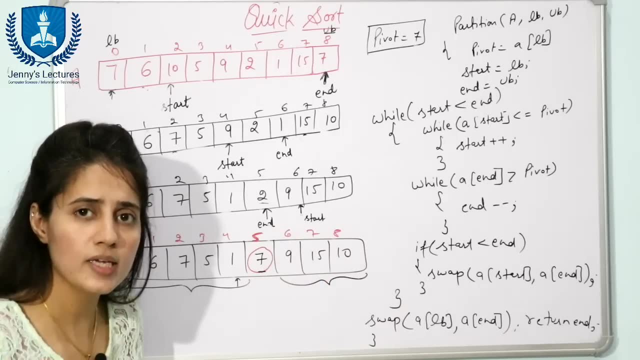 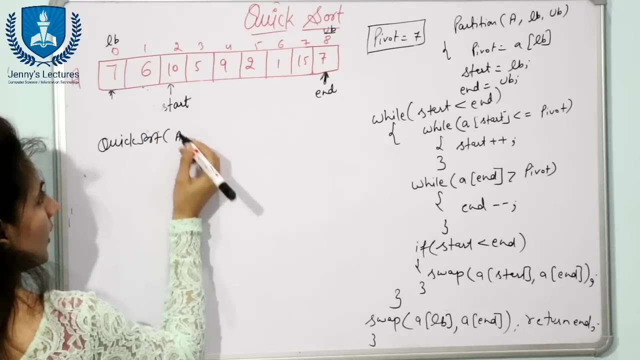 to this return, this end, this position. fine, now, this is the main, this is the backbone of this quick sort algorithm. now, how to write down the quick sort algorithm? that is very easy see. in quick sort we have one function. we are going to supply this array- lower bound and upper bound- fine, 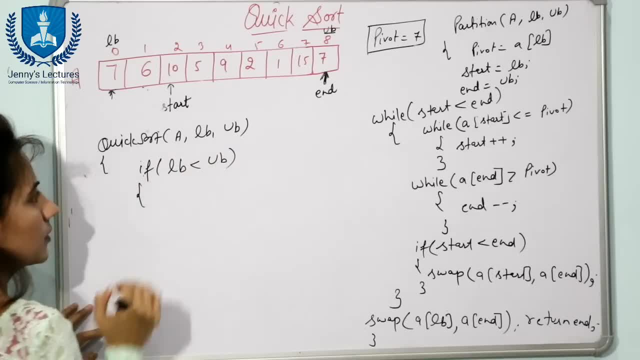 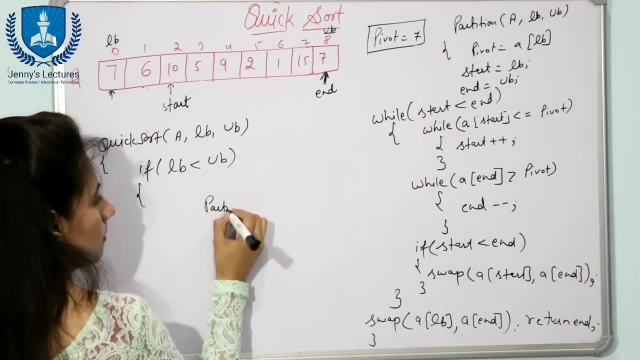 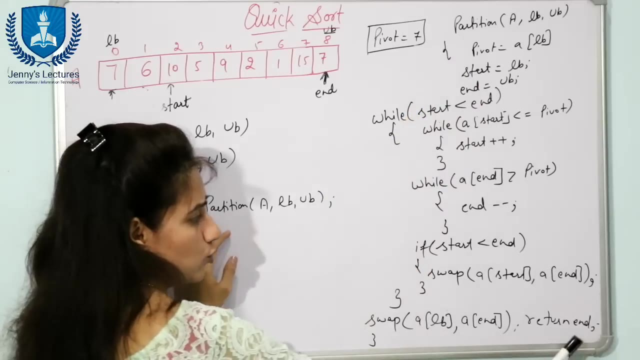 and if lower bound is less than upper bound, then you will do what you will. you will call this partition function partition a of lower bound and upper bound. this partition function is going to return this end. that is something you can say. location you can say. so here you are going to.